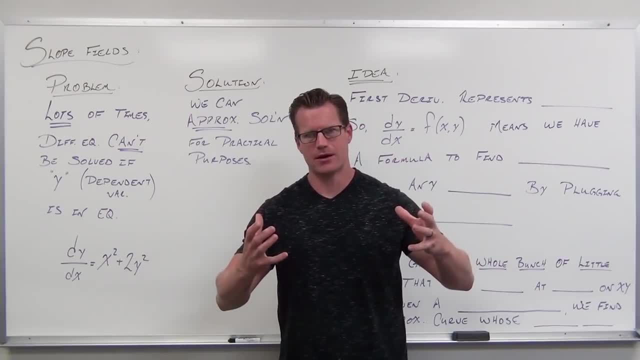 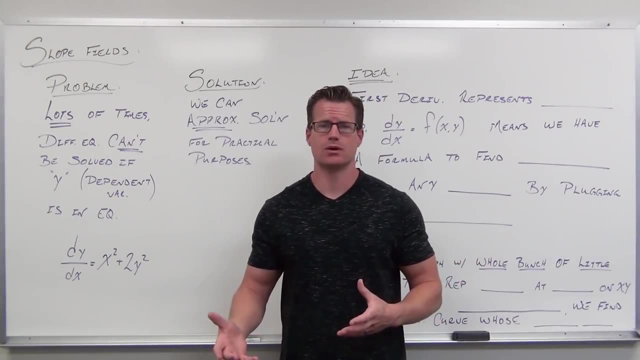 we might have slope fields and this kind of breaking the pattern in our heads that we have to have an exact solution all the time in real life, Because that's not true. So a lot of differential equations use approximations because there aren't any good techniques to solve some of these things. we're going. 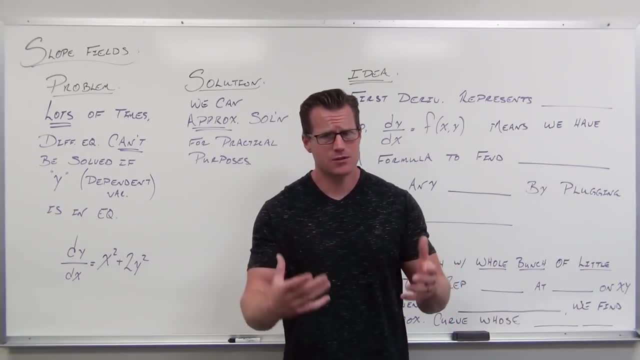 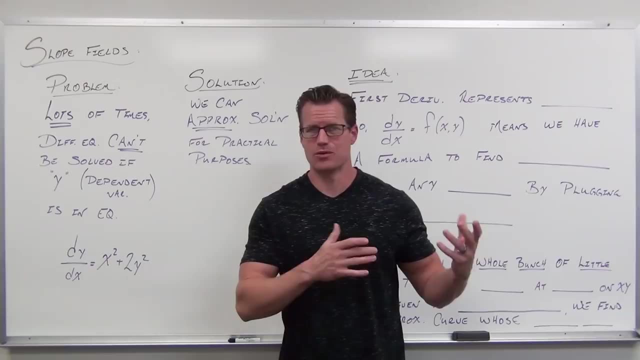 to come up against. That's one of the ideas of slope fields. So in this video, what I want to get at is what a slope field is, how a slope field can help us identify a solution even if we can't explicitly define it, And that's. 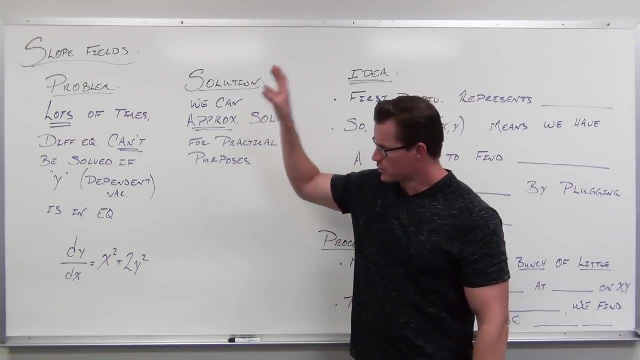 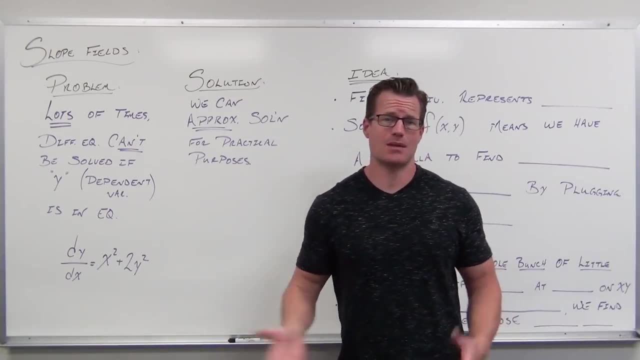 important. So here's a slope field. They'll go through a problem, a solution, an idea and a process of how we're gonna go about it. So here's the problem. Lots of times, differential equations can't be solved if they have this dependent. 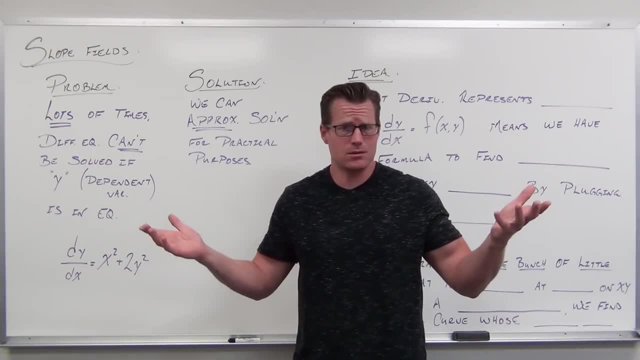 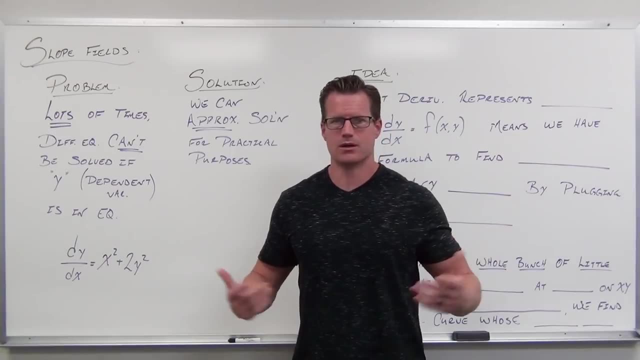 variable y in them. You look at it and you go: there's nothing we have. It's not separable. We'll talk about separable. It's not linear, Talk about linear. It's not exact a substitution we can make. It's not homogeneous. Well, I don't understand those things. You're not. 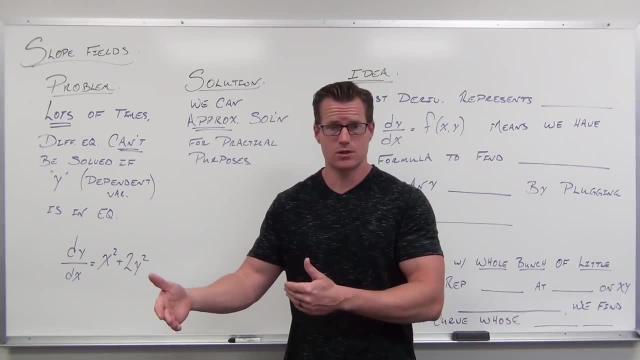 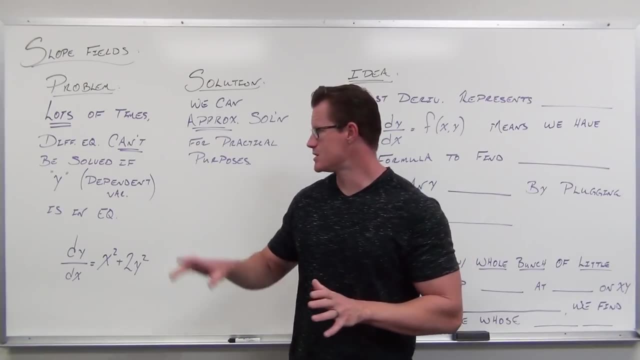 supposed to right now, but we're going to get to those techniques of solving differential equations as we move forward, So don't worry about it. But the point right now is that sometimes we come across these differential equations that have y in them that we're not going to be able to do. 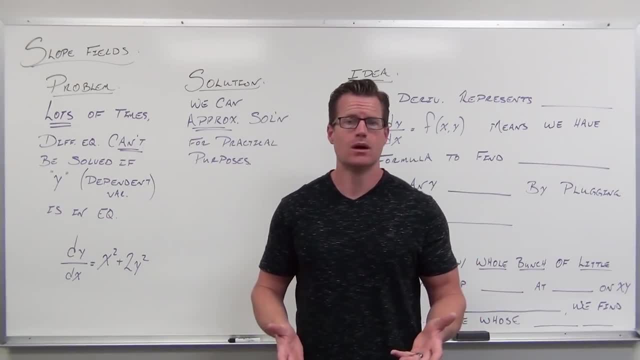 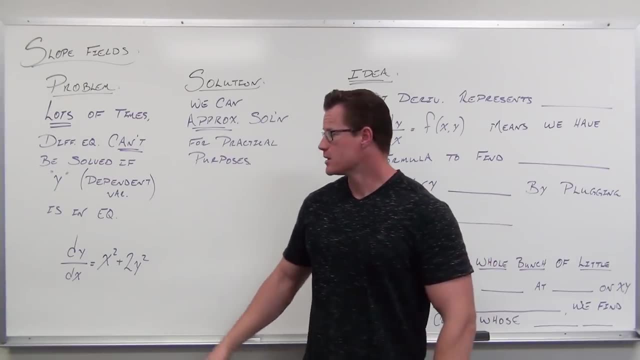 anything with. And you look at it and you go: there's nothing I can do. So what's a possible solution to that? That's what a slope field and some other techniques help us with. So here's an example of the derivative of y with respect to x. So a differential equation has a first. 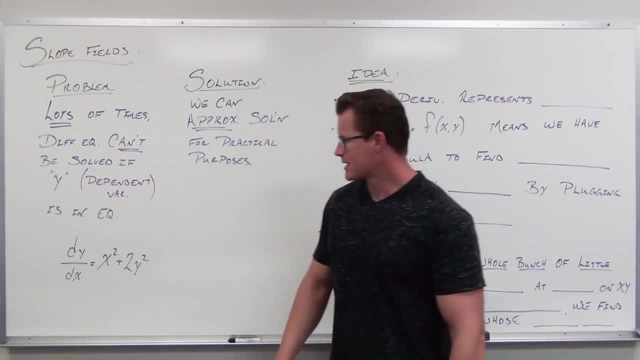 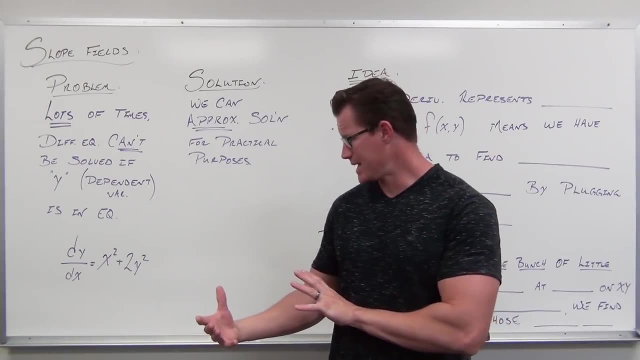 derivative. a first order differential equation has x squared plus 2y squared And we go: that's got a y in it. There's nothing that we know of that's going to help us to solve that. There's nothing to do. So sometimes you run into that in differential equations where there's 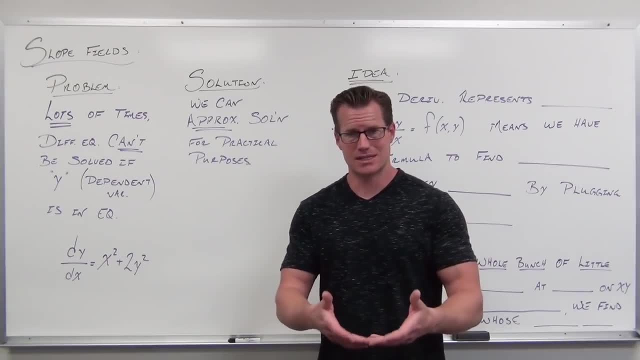 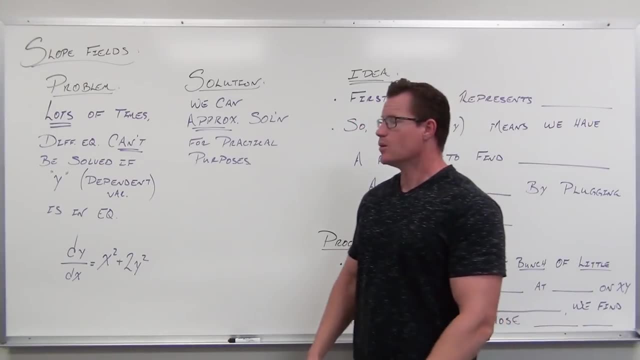 nothing that we can do to get an exact answer, an exact solution. So that's what a slope field and some other techniques help us with: General solution or even a particular solution that's going to fit that. So one solution to our problem is we can oftentimes approximate solutions and that works for some practical purposes. 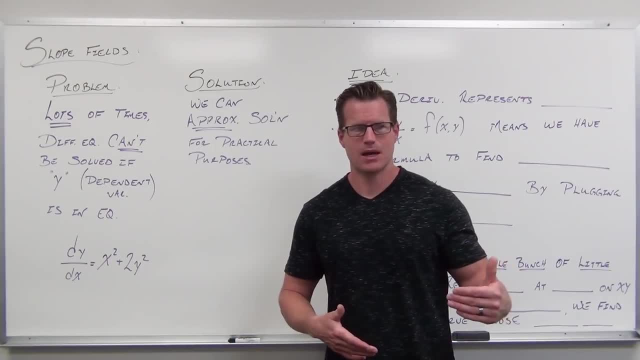 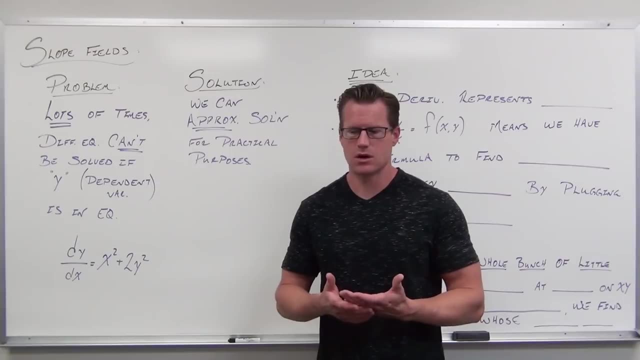 And a lot of people in math when they get here they don't like that. I didn't like it. I still don't really like it, that there's not a solution. You know, when we have linear equations, you solve it and you get one answer, or you get no solution or infinite solutions, But we get. 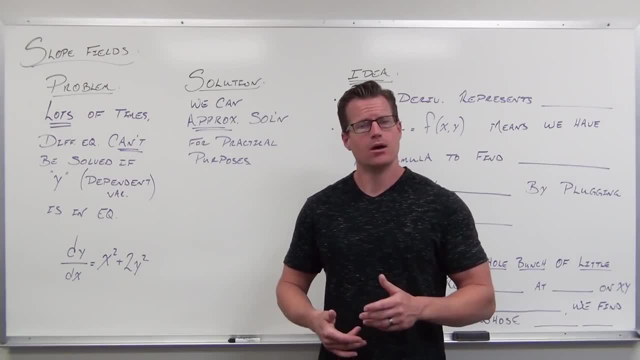 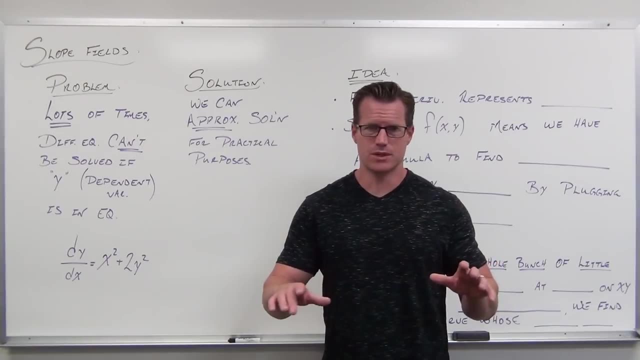 and answer, And there's a process to doing that Well, with a differential equation. sometimes there's not, And so we have to get kind of used to this idea that not all the time do we get the answer that we're looking for, by a process that's outlined like step one, step two, step. 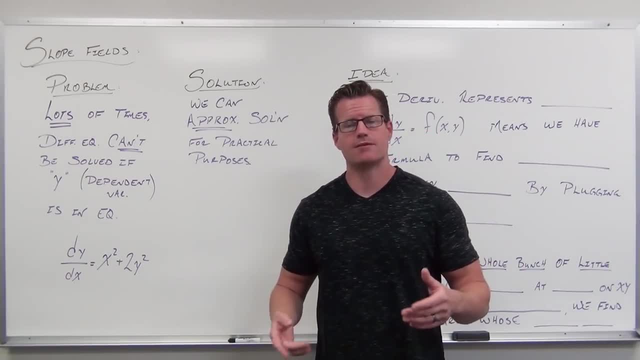 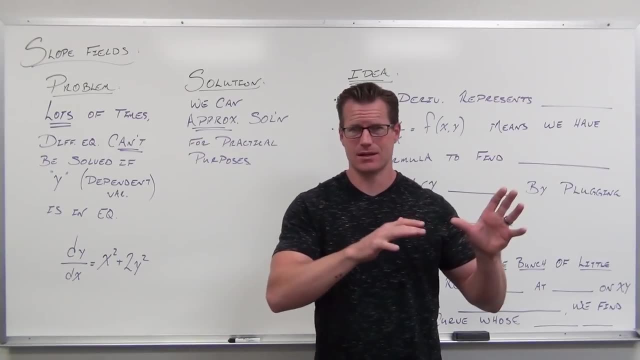 three: It doesn't exist in some cases. So we have these techniques to approximate and it works in real life really well. So we say, well, while we can't find an actual solution, we can approximate it. It's going to work just fine. 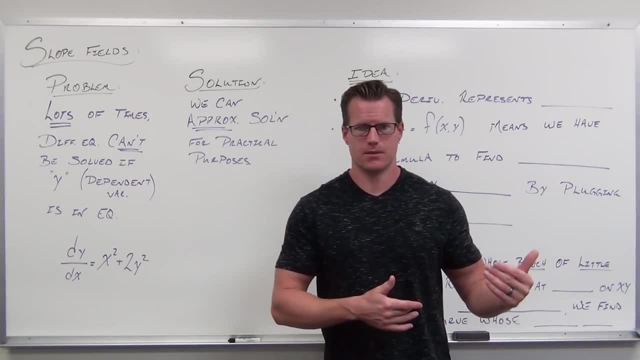 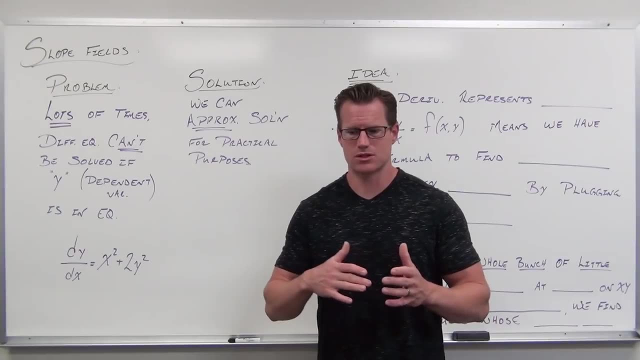 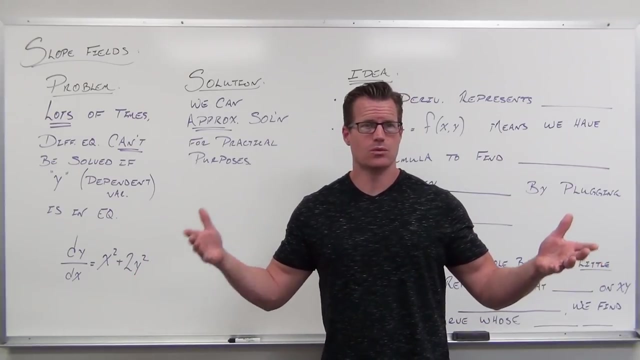 And, if you remember, we talked about that a few videos ago, where we said that these approximations are good enough, that these approximations are something that we can model life on, And when we get too advanced in our equations, we can't solve them anyway. So 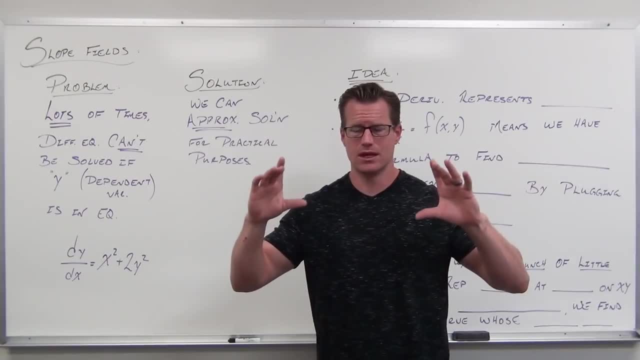 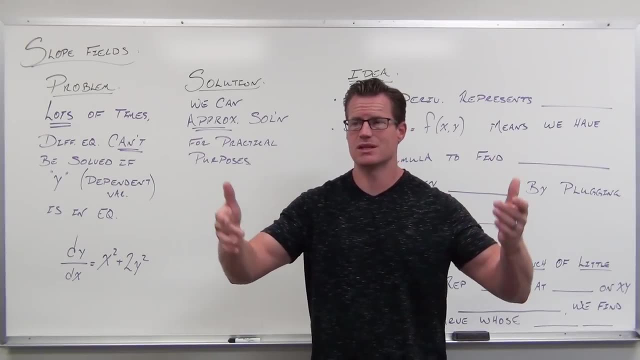 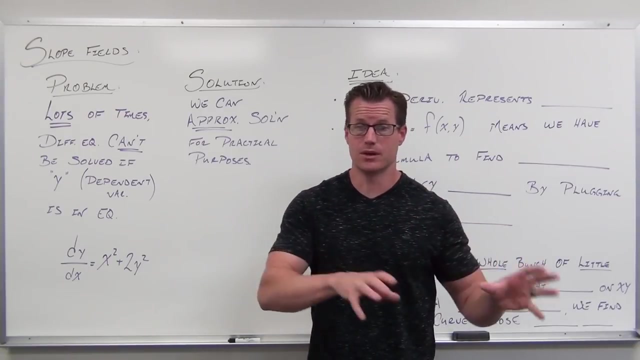 we have this trade-off: If we start limiting variables, well then we are not perfectly representing our situation. But if we perfectly represent our situation, then we can't solve it. So sometimes, in making an equation better, we limit our ability to solve it. And that's where 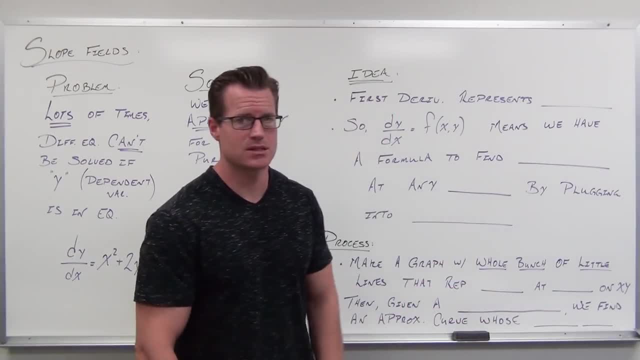 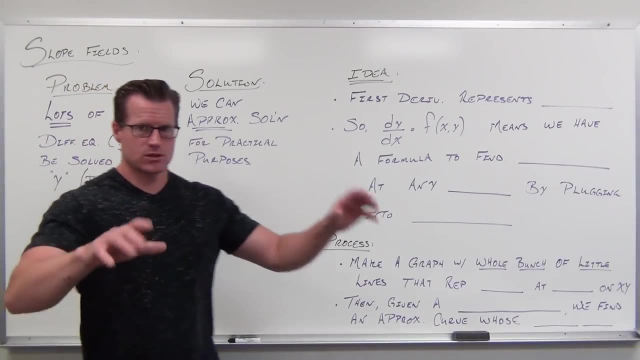 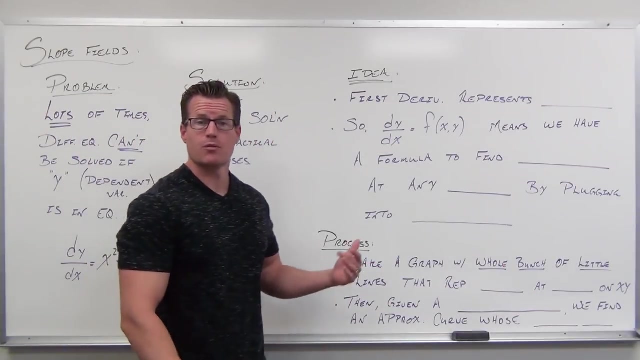 approximations can come in and help us and say, well, I can't particularly solve this, but it's good enough for the real life application I'm trying to represent. So here's the idea. So again, sometimes you can't solve it with the techniques I'm going to teach you. Here's a solution We have. 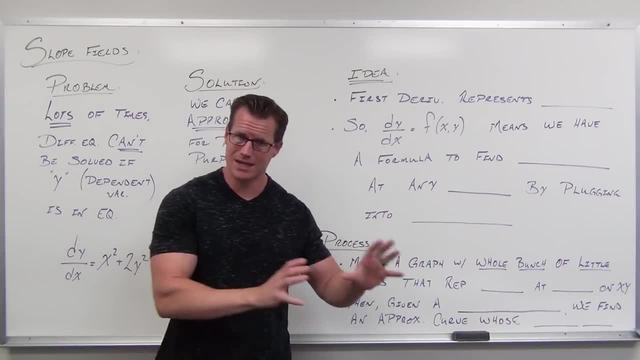 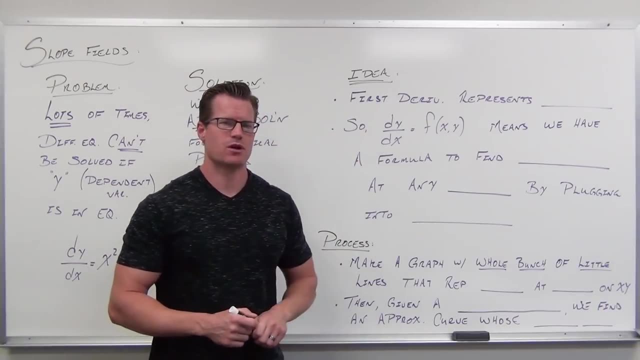 approximations. Here's the idea on how to get that approximation. One idea is called a slope field. So here's what this idea does. If we know that first derivatives represent slopes, we know that a derivative is a rate of change. A first derivative represents a slope of a function. 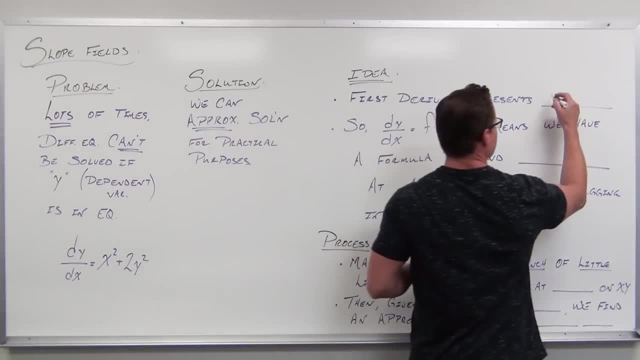 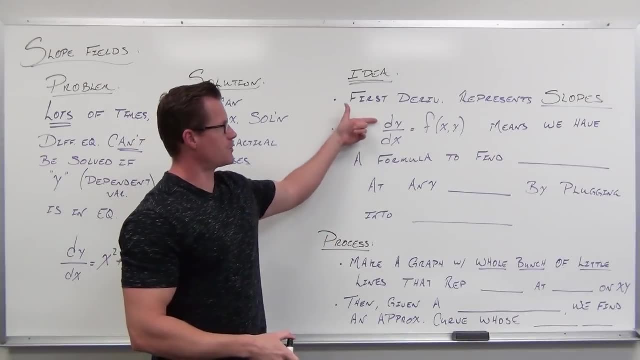 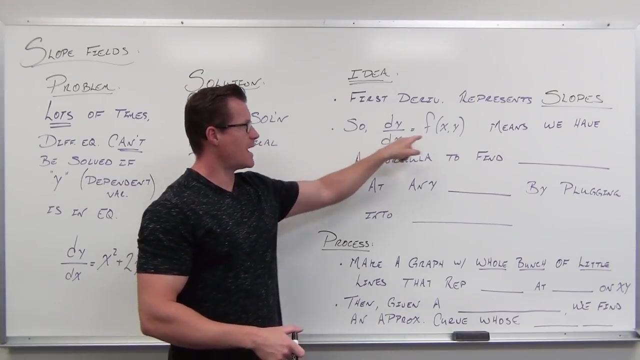 that we're dealing with. So a first derivative represents slopes. So if we have a first derivative, a derivative of y with respect to x, derivative of the dependent variable with respect to the independent variable, if we have that slope field we're going to have a slope of x. So if we have a 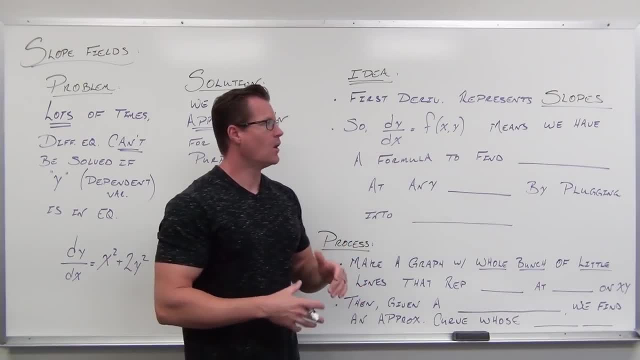 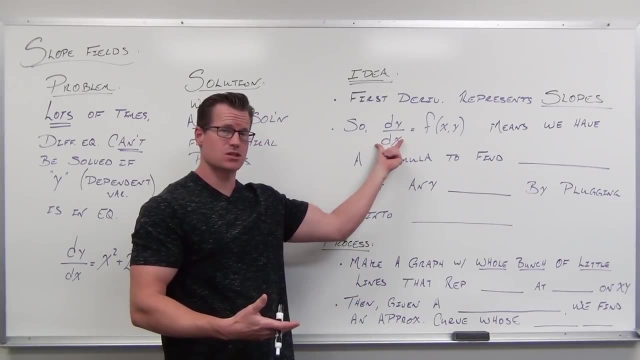 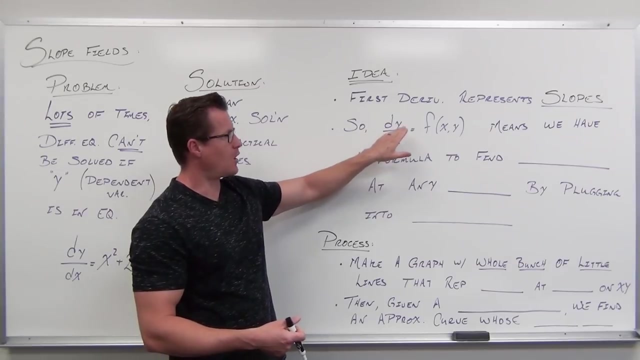 solve for some function that has both x's and y's in it. What that means is we have a formula to find the slope. That's kind of cool. This represents the slope. So if this is the first derivative, this is the slope. that's our formula. So our first derivative, our slope, is represented. 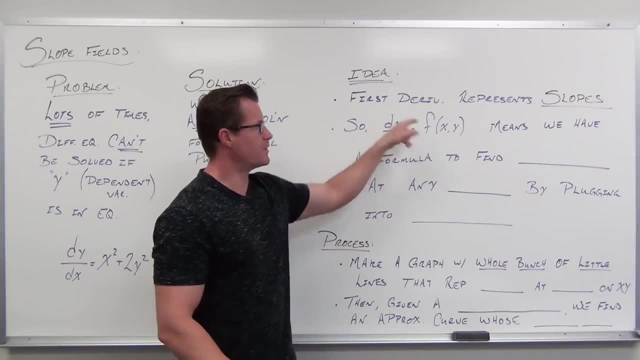 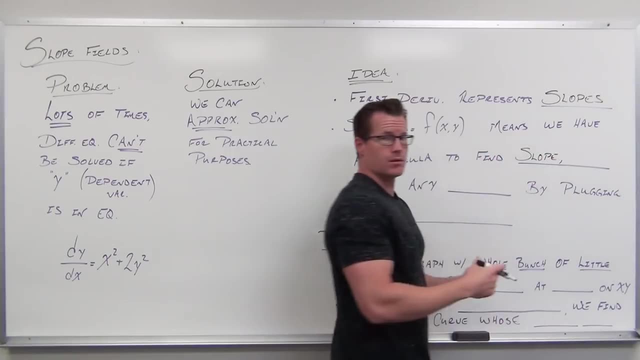 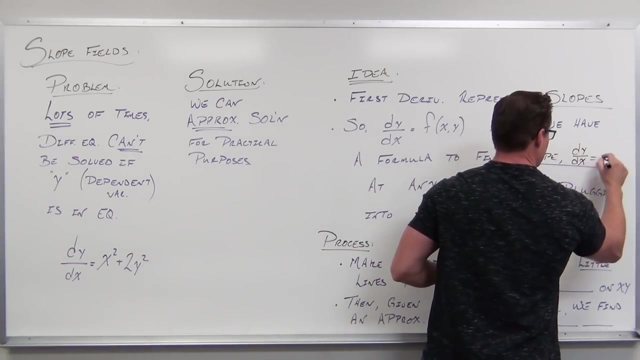 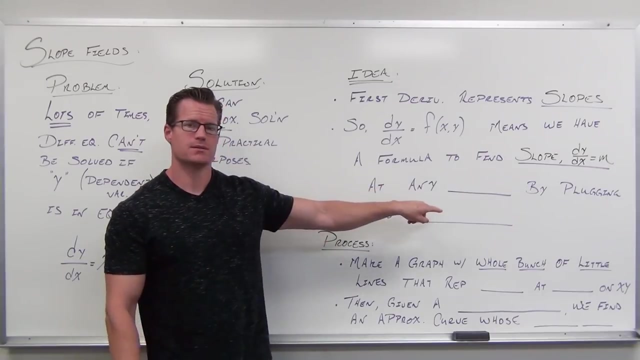 by this formula with x's and y's. That's neat. So this means that we have a formula to find our slope. More specifically, this represents slope. So the first derivative represents slope. So we have a formula to find the slope at any point, at any point that we want to. Why, Why? 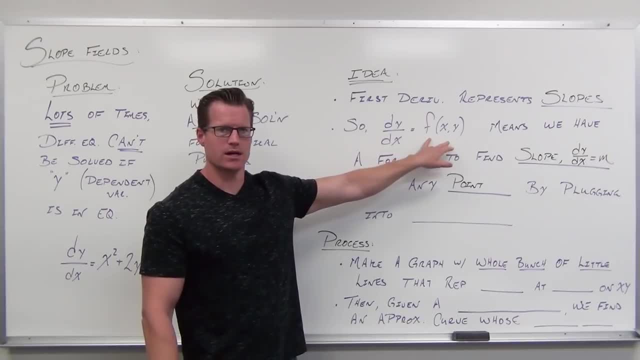 does that work? Well, if this is our slope and it's based on x's and y's, points have an x and y origin, so it's going to radiate over the x's and y's and therefore have a AND Scripture. 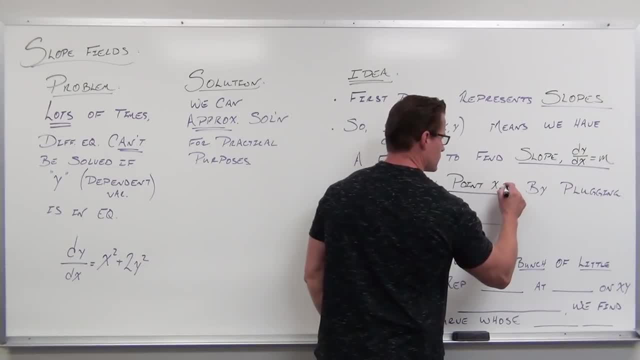 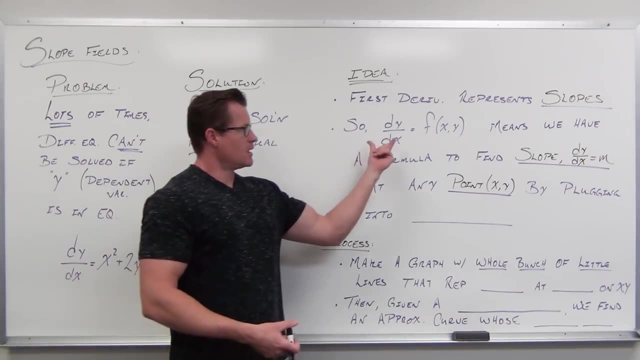 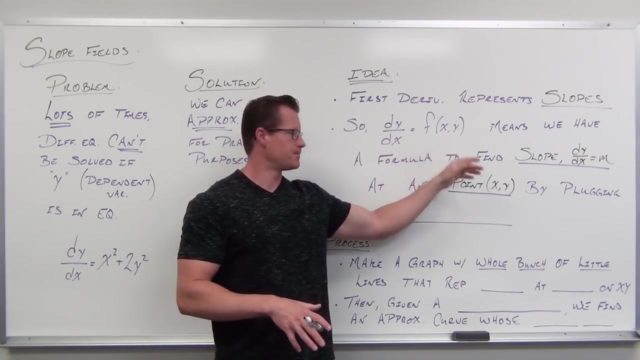 It's got an x-coordinate and a y-coordinate by just plugging it into the function And that should be pretty straightforward to us. If a first derivative means slope and this slope equals some function in x and y, given any point boom x and y- we can plug that point into this function and find a slope. 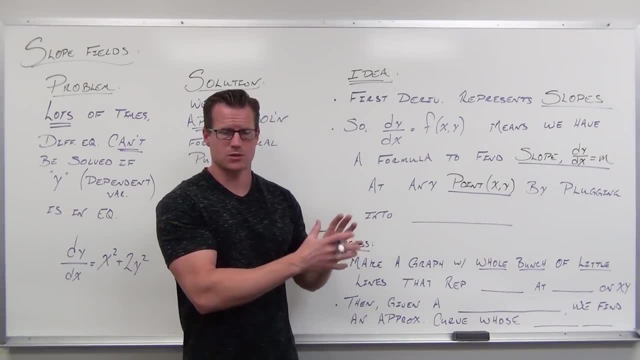 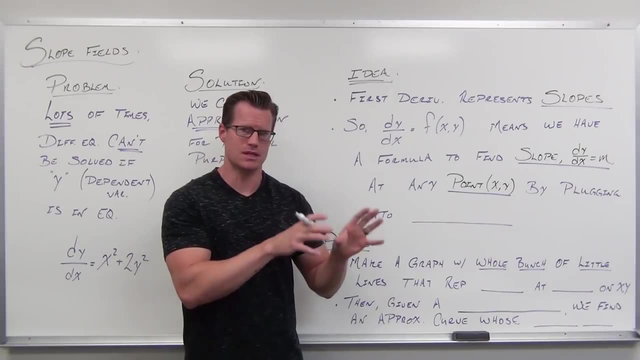 at that point, provided that it's continuous at that point. So provided that we're not at an end point, provided that we don't have a gap or a hole or it's not defined, So that's important. We'll get into uniqueness and existence a little bit later. two videos from now. 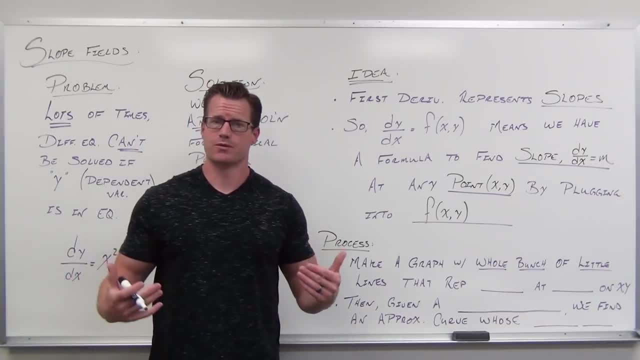 So short recap, we're almost done. I'm going to get to two examples to show you what slope fields are. They take a while to create. They're not hard. A lot of people use computer graphing to do this, or a calculator. 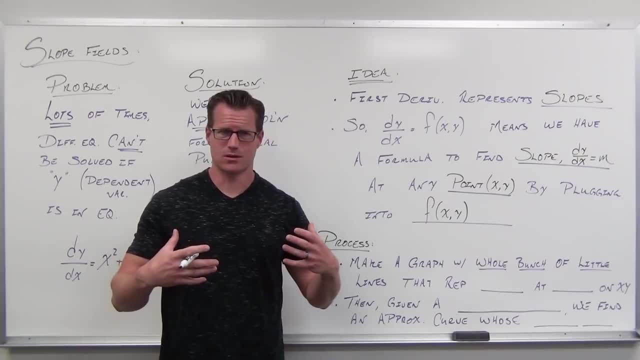 I'm not going to be showing you that, But of course my ideas here are to get you to understand the concept, Not just to be able to do it, but to understand what's going on, And I like to do that by hand when I go through this. 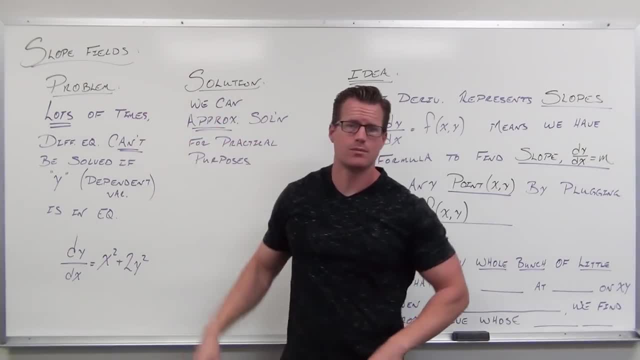 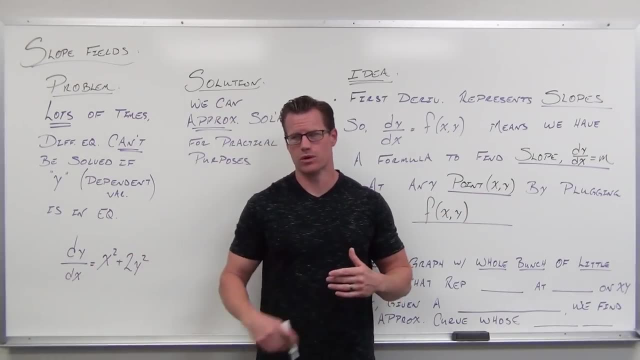 So slope fields problem: we can't solve them all. Solution: maybe we can approximate them. One idea is: hey, if derivatives represent slopes and you have a differential equation with a derivative in it and we can solve it for a function of x and y, then we have: 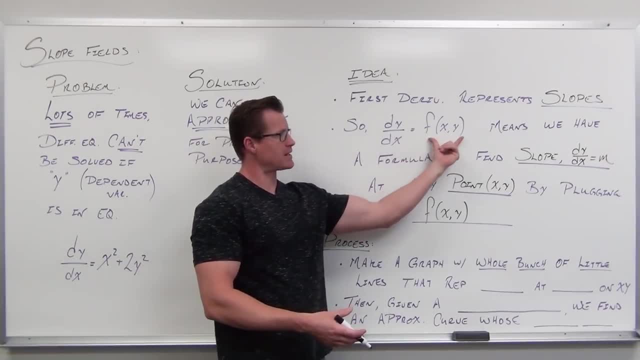 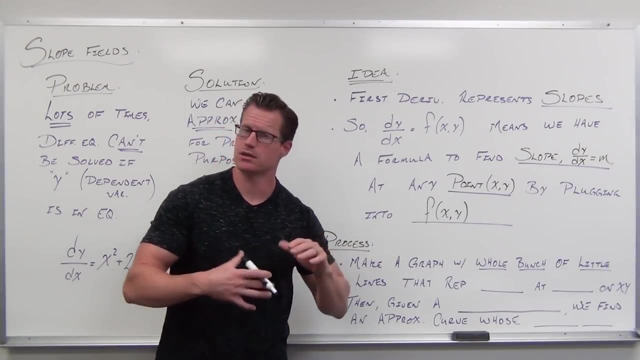 a formula to find slope at any point. This is slope. That's the formula. Just plug in the point to our function and you're going to find the slope at whatever point x and y you just plugged in. So here's our process. 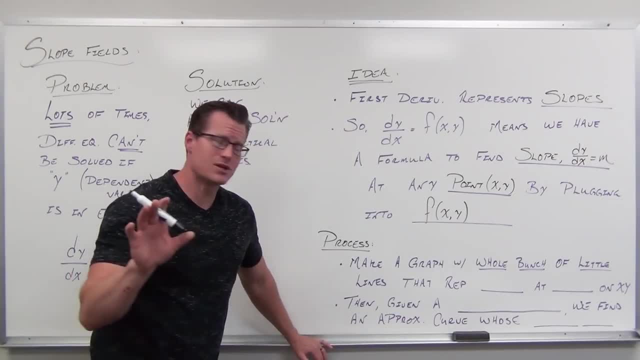 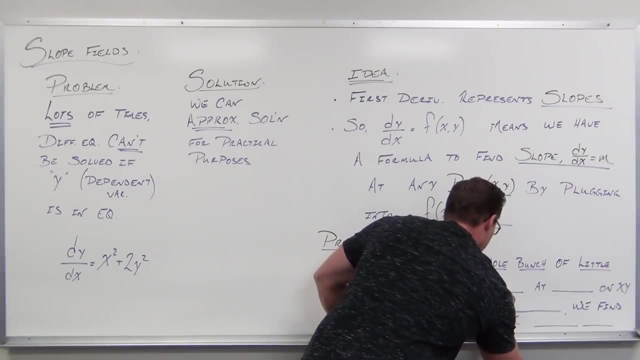 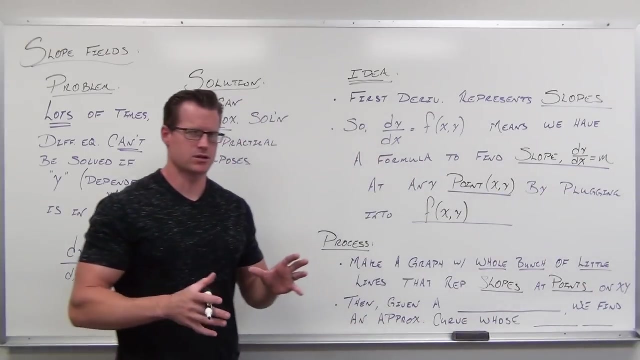 What we're going to do is we're going to look at this. We're going to make a whole bunch of little lines that represent slopes at points on the x-y plane. It's not as hard as you might think, because you're going to have tons of slopes, but there's 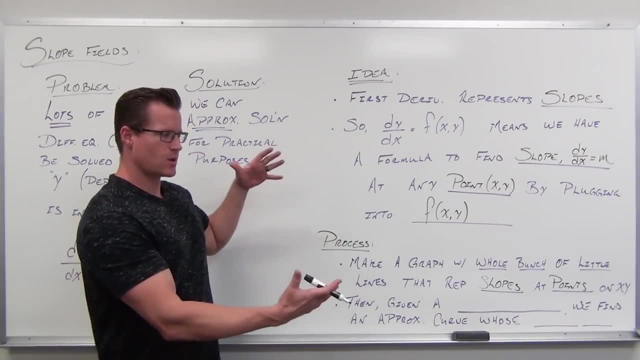 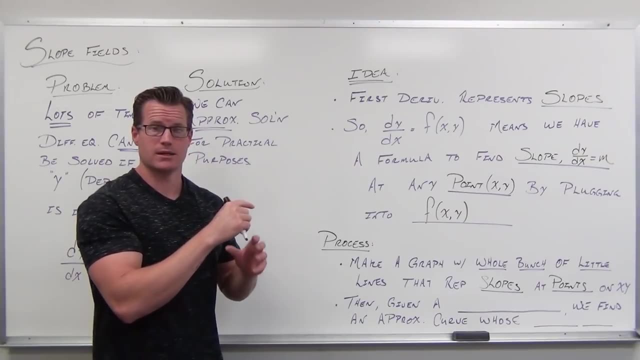 a pattern to it. I'm going to show you. So make a graph x-y plane that has a lot of lines. It's going to represent little slopes, So they look like unit vectors, almost without the arrow. If you've had Calc 3 and you've had vectors, so you see those little unit vectors all over. 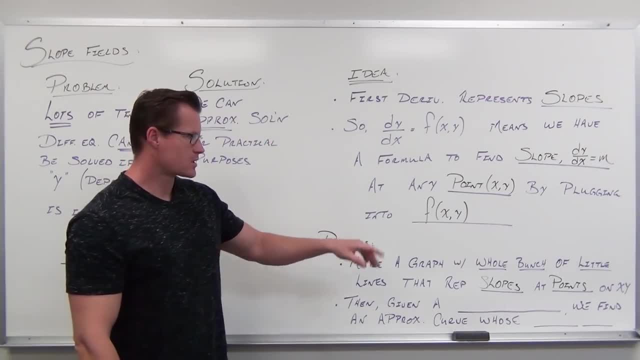 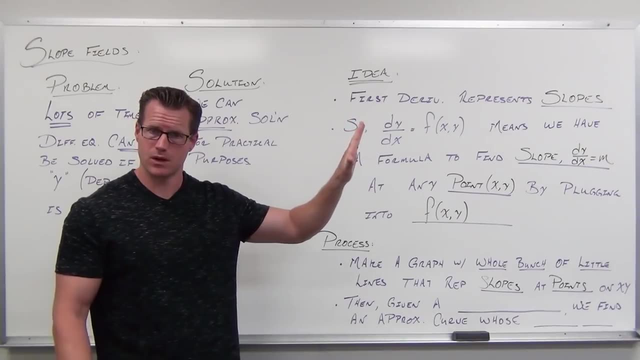 the place. they really look like that without the arrows At points on x-y. they just give a direction that your line is going. Well, that's what slope does, right, It gives the rate of change at any point on a function. 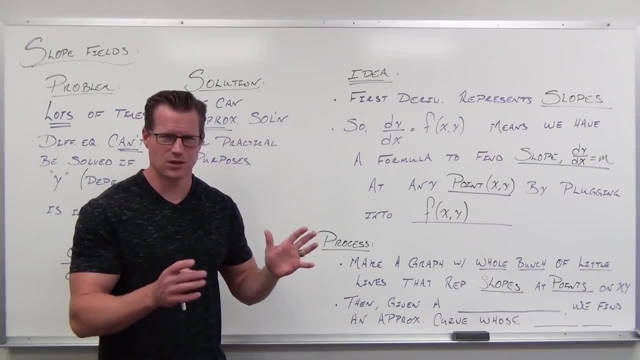 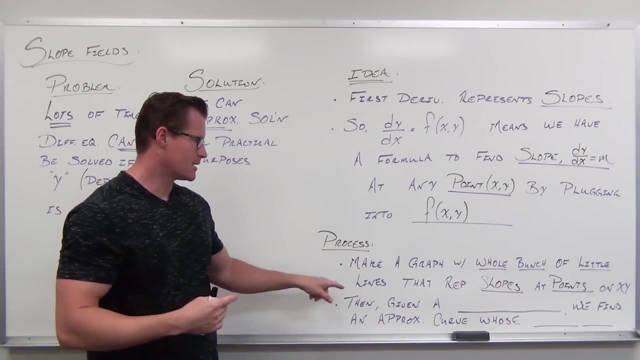 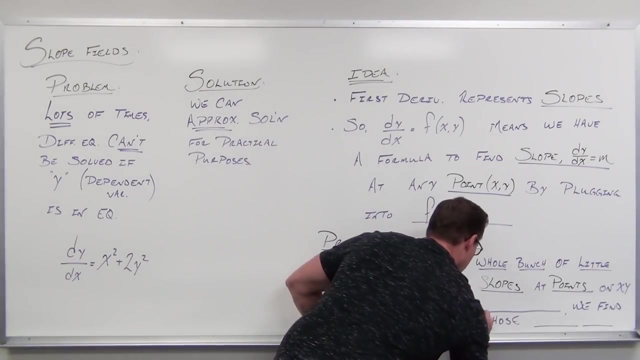 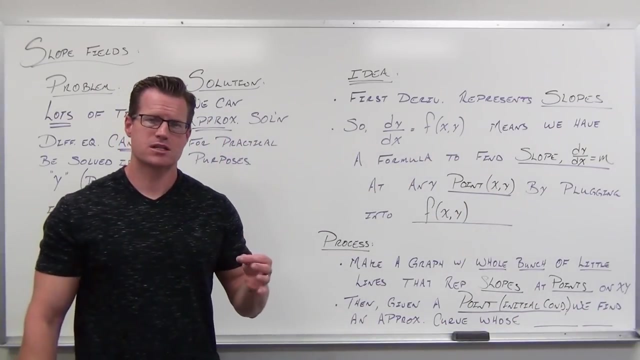 And so our idea is: if we make this graph with a whole bunch of little lines that say, hey, at this point the function should be going like this, Well then we can put all of that together And, given a specific point, an initial condition, then we can find an approximate curve whose 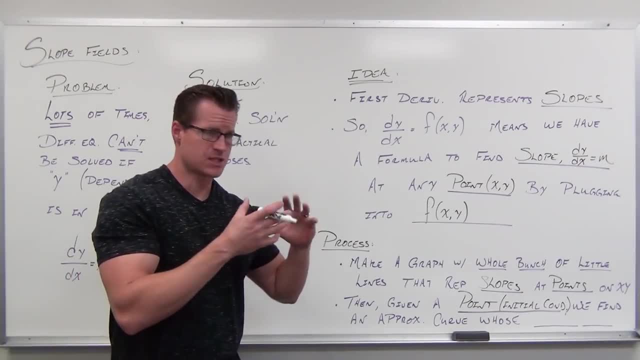 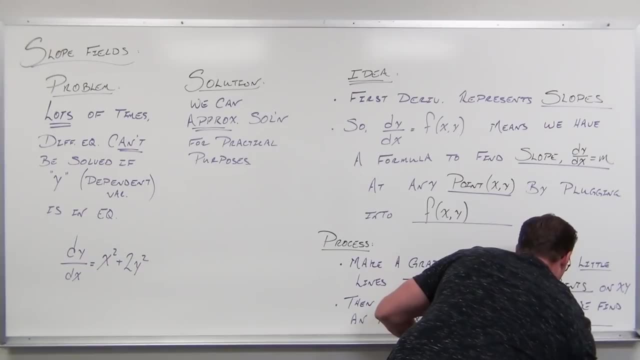 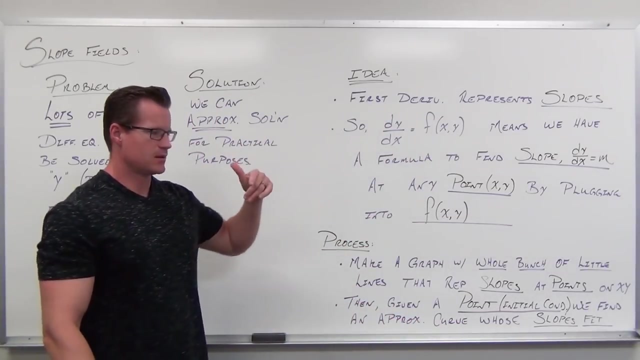 slopes fit that field accurately At every point. whose slopes fit, And what we mean by that is it is this. So here's the general idea, and it's going to seem vague because we haven't had any examples, But here's the idea. 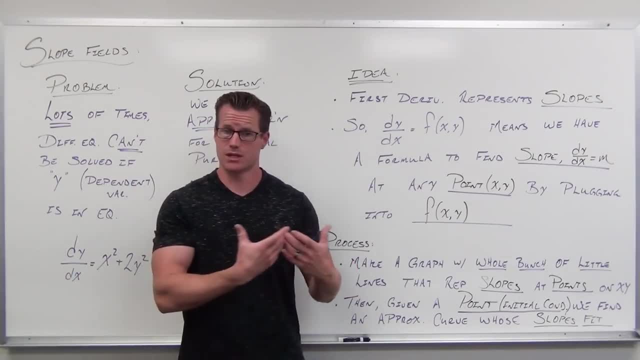 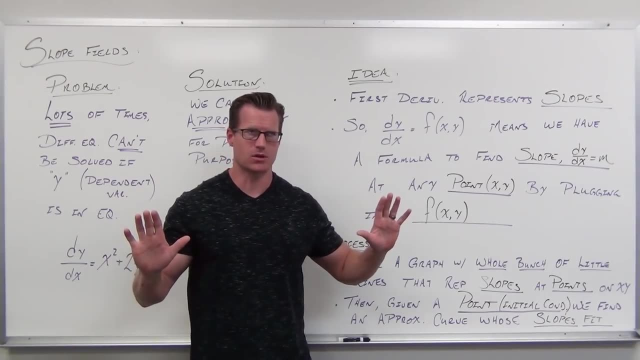 You're going to take this function, this differential equation that represents slope- Slope is the first derivative- And you're going to take every point on the x-y plane- And that sounds hard- Take every point and plug it in And say, well, at this point I get this slope. 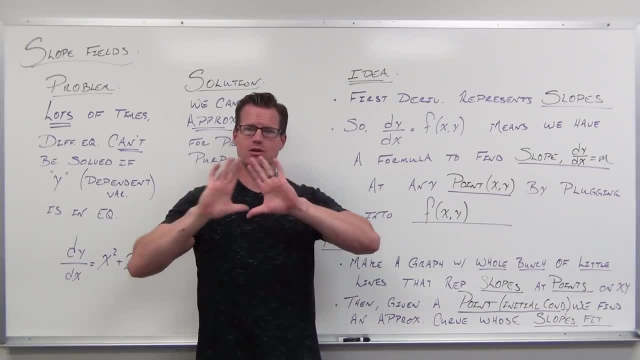 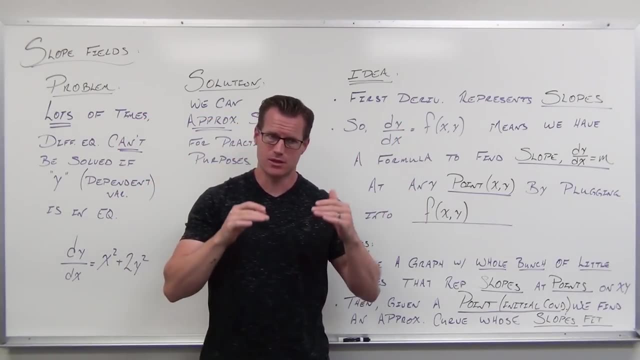 At this point I get this slope. At this point I get this slope, And you're going to make this huge x-y plane. There's going to be slopes everywhere, These little lines that represent direction at every point. The slope can be given at any point just by plugging it in. 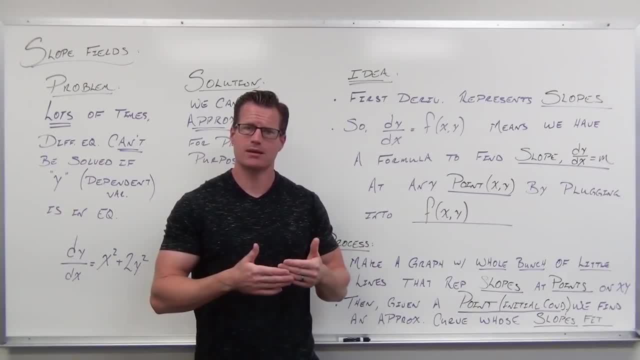 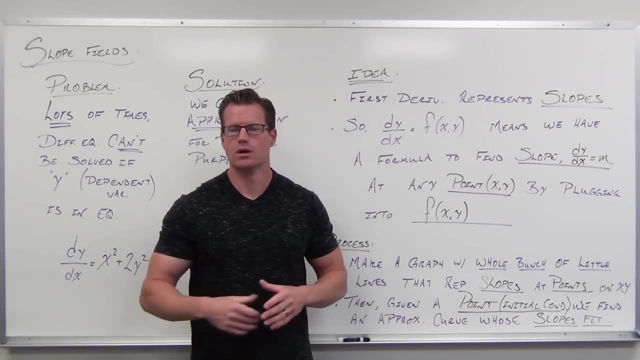 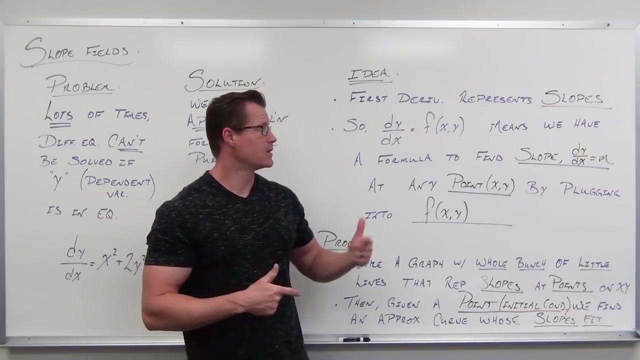 So with the whole x-y plane we could potentially plug in every point. Can't plug in every point, But like the point, The point, We can find the slope for any of those points where we have a defined function. So where it's continuous, where it's differentiable, we can find the slope of. 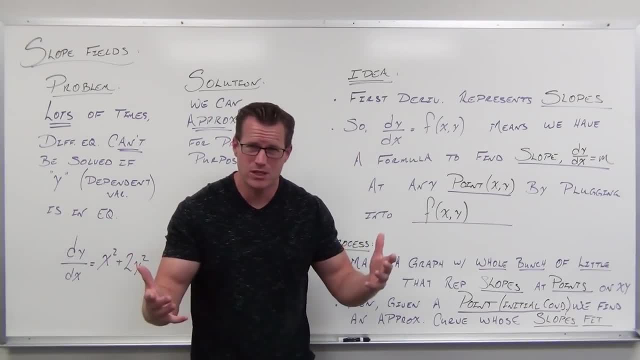 So we're going to do that. We're going to take the whole x-y plane, We're going to take every point on it that we can find And we're going to find the slope of those points. It's going to look crazy. 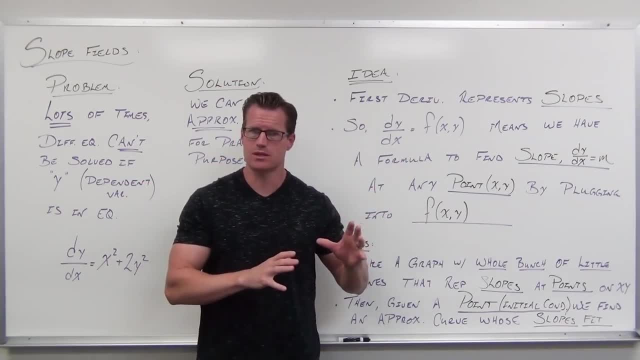 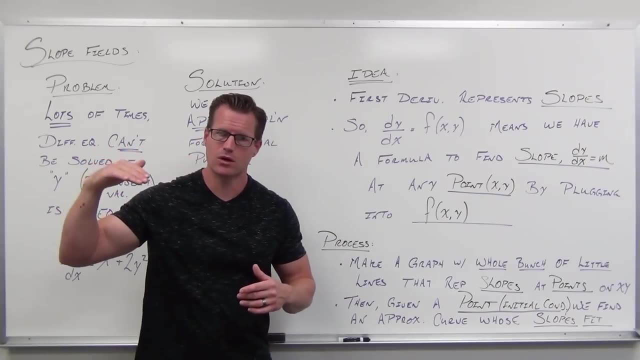 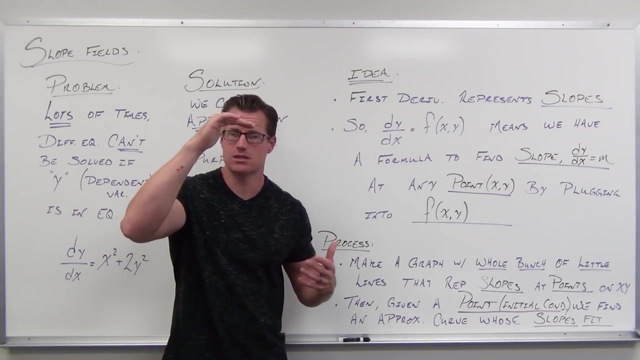 We have all these little directions, all these little slopes on this plane. Then if I give a specific point, well we can say: this is the way the curve has to go, Or has to travel to make it through that point and to fit all of these slopes. 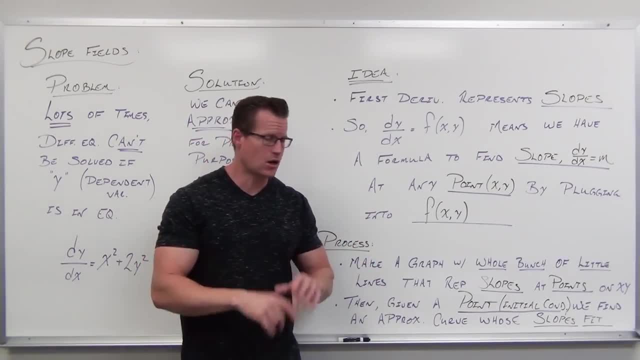 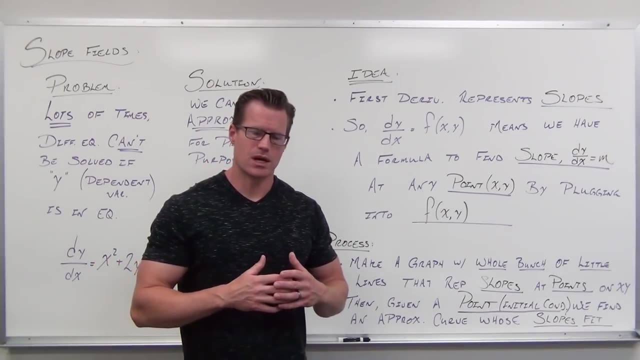 So, given a point or an initial condition- that's what we're talking about- Then we can start approximating the curve. So here's what you need to know about these slope fields that we're going to create. When we create a slope field, 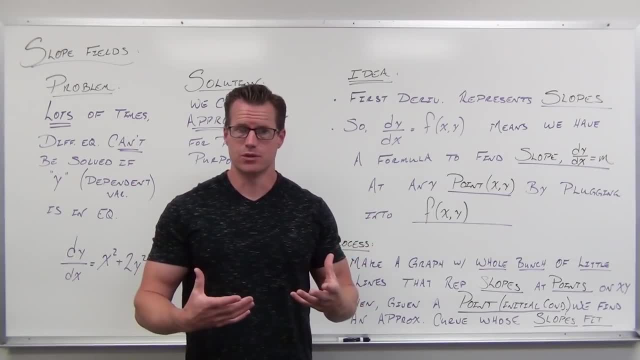 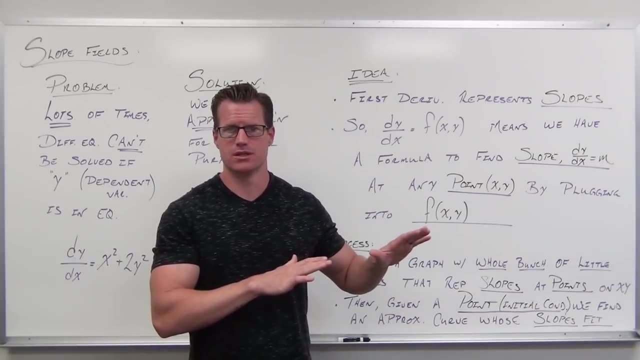 So all these slopes on the plane? It's a general solution. It says that this is everything that could happen. These are how all the curves would have to look to go through these slopes, To make sure that we're fitting the slope at every single point. 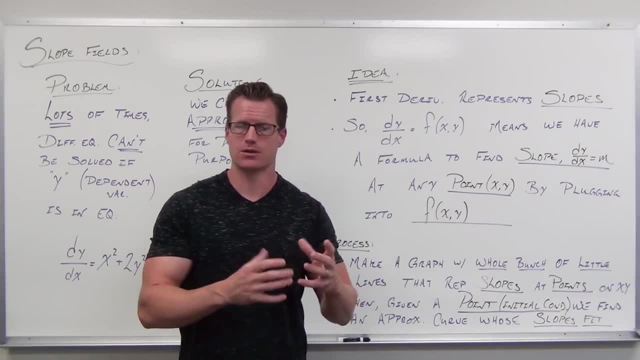 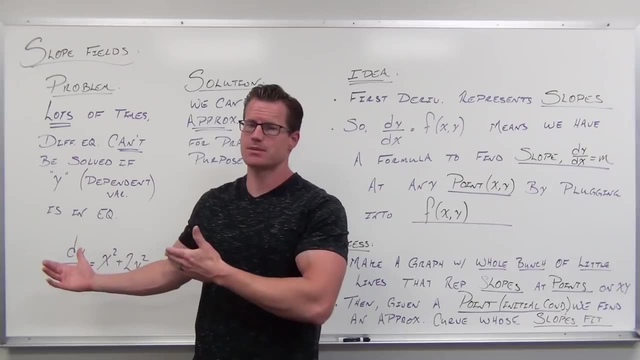 If you want one specific curve, a particular solution, like we studied before, You need an initial condition. You need a point to go through. So long story made short. Sometimes stuff don't work. We need approximations. One way is to find the slope at every point. 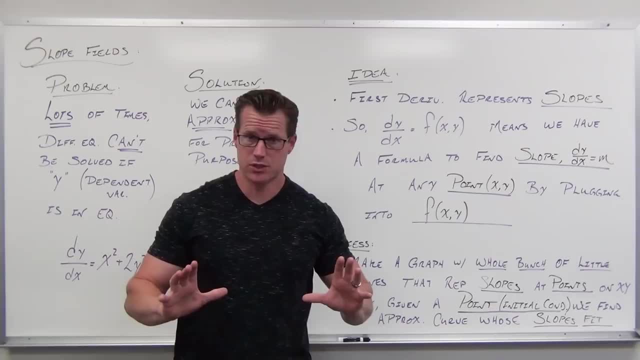 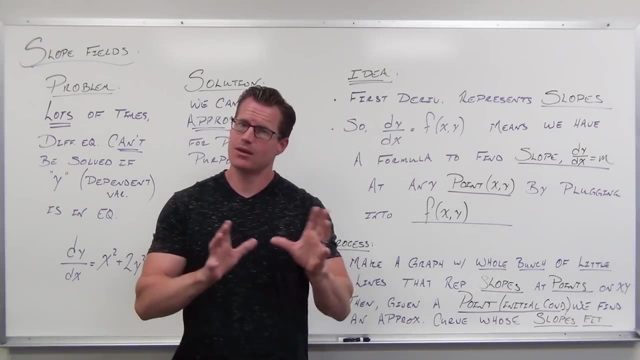 Put it on a graph And then that represents your general solution. That represents all the curves that would have such slopes, That would have such slopes. Then what we do is we say: if we want a specific one, you just need a point. 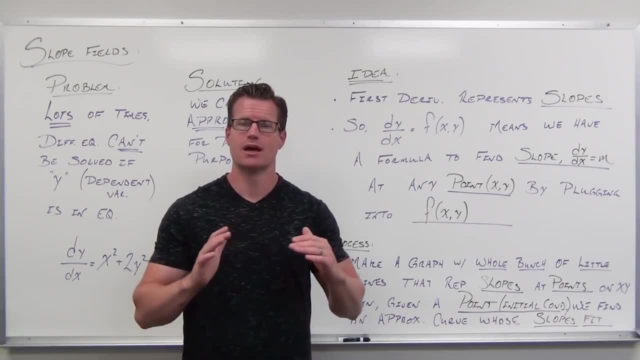 And that will limit the curve. So we'll find a particular solution that fits on our slope field, That also goes through that point, And at every point along that curve we're fitting the slopes. That's the idea. Well, what I want to do now is show you two examples on how to create them. 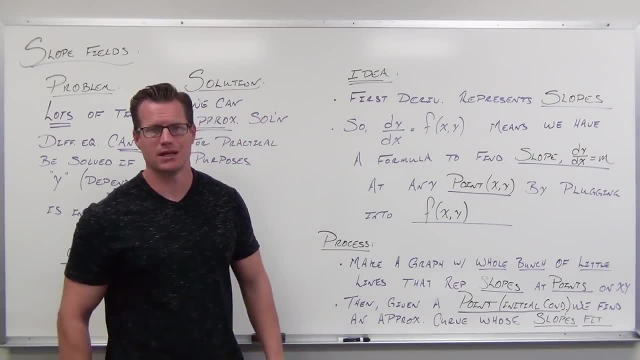 And then all of this is going to make a lot more sense, Because, as we go through it, I'll be explaining: Hey, remember how this makes slope, And remember how we need a point. And now we can go ahead and see a specific curve. 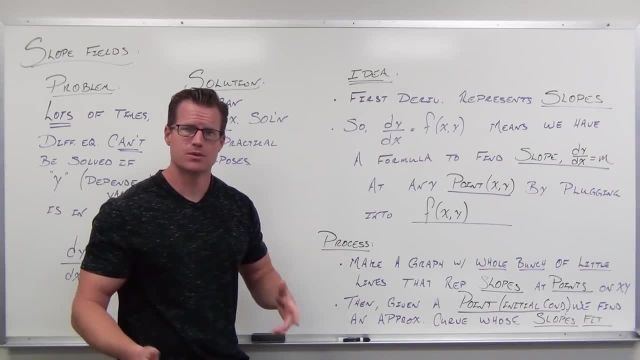 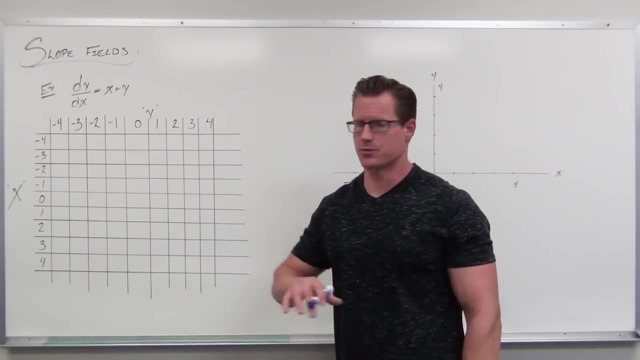 So I'm going to do that. We'll do just two examples And I'll walk you through how to do that. So let's get started on our example. We're going to build a slope field from scratch. So no computers, no calculators. 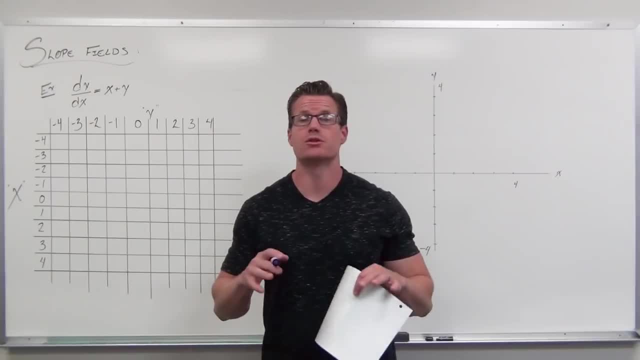 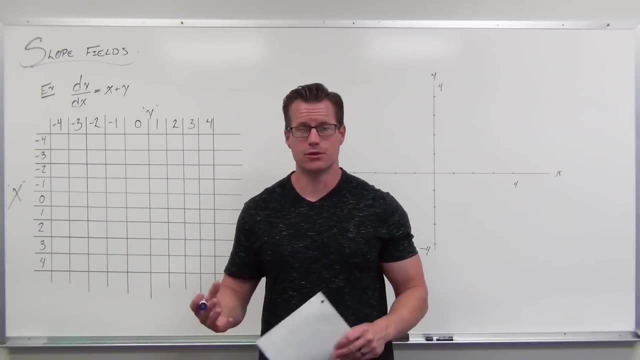 Because I want you to understand what's going on here. They'll do it for you And I'm sure that you're going to use it in whatever class you're in. You can get a computer And that's a great way to build slope fields when you have some difficult differential equations. 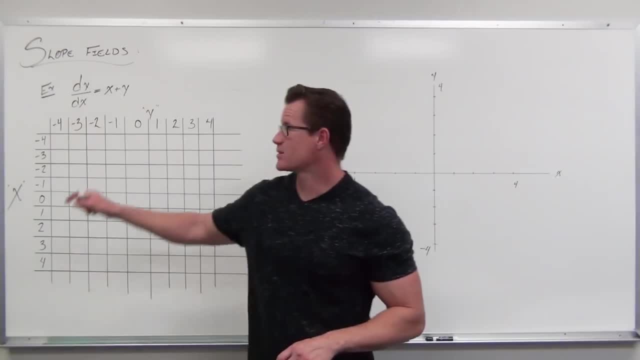 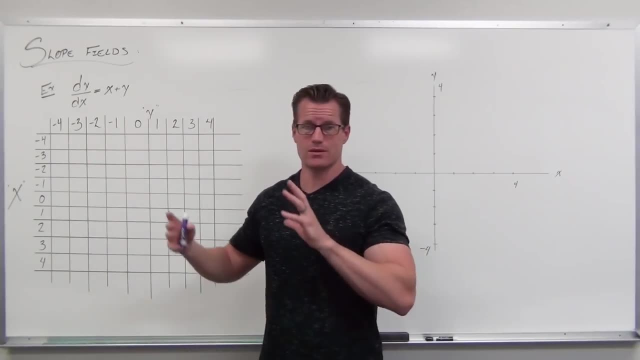 So here's our problem again. Sometimes these things aren't solvable. I'm not saying this one's not, I'm saying I'm giving you an easy example here so we can see what a slope field does. So whether there's a technique or not to solve that explicitly, I don't care right now. 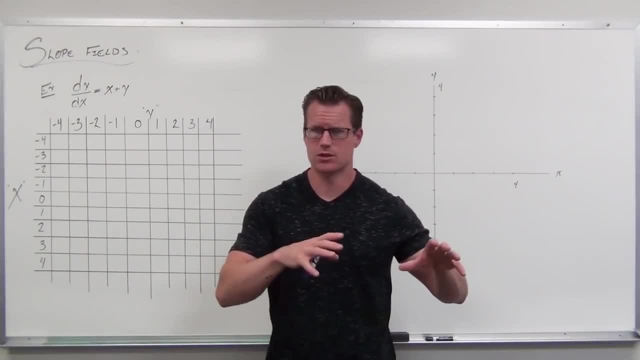 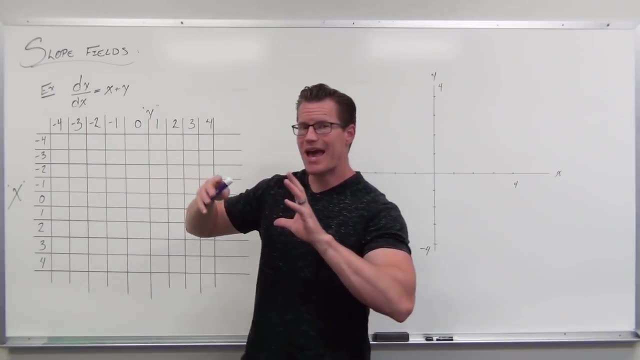 What I want is your idea of slope fields to be built in your head so you understand how they work. So here's our point. If that right there means a slope, then that's the formula for the slope. So at every single point that we have x, comma, y, we can find the slope. at that point of our general solution. 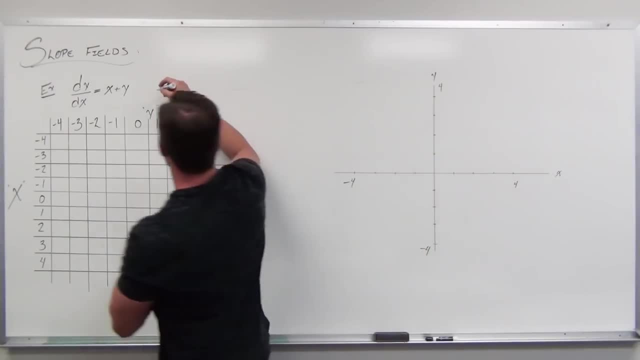 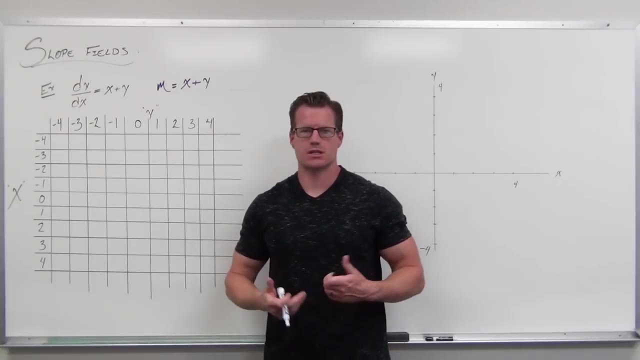 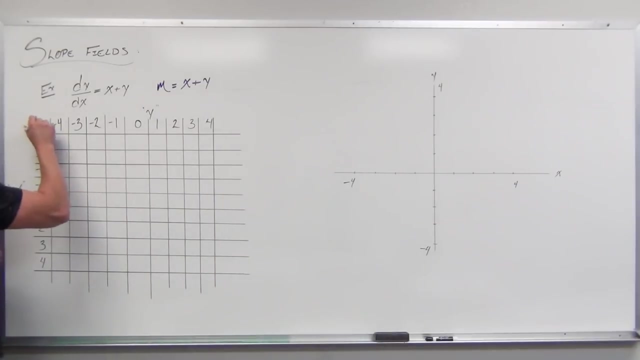 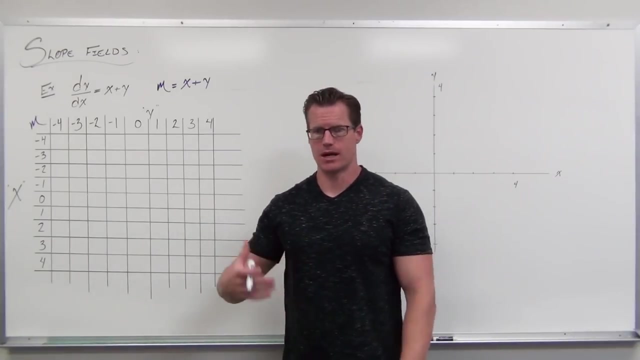 Whatever curve is going to fit this. So our slope first derivative is just x plus y. That means that if we have our y values and our x values, we can make a table for slope really really easily. All we do is we have to add up our x plus our y value. 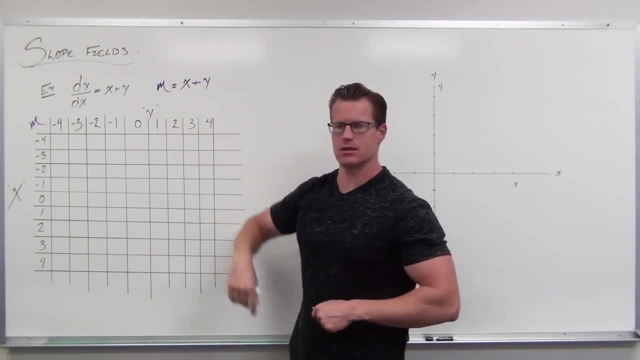 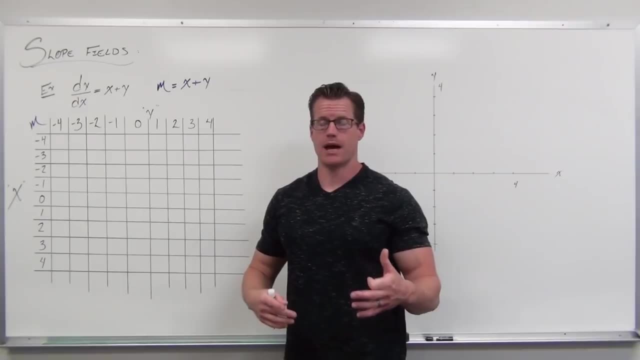 So say, take the x value plus the y value. It's going to give you the slope. We're going to make a table up like that. It looks like it's going to take a long time, but there's a lot of good patterns here. 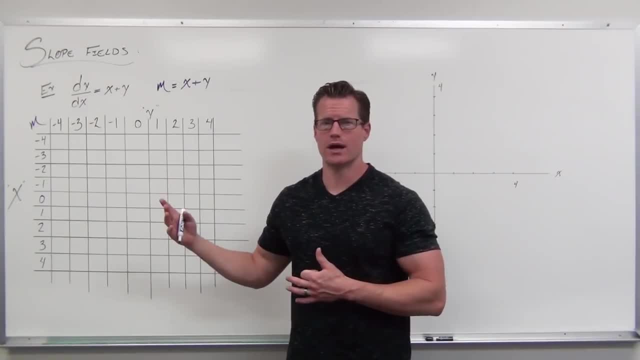 So I'm going to show you how to find the patterns. I'm going to show you how to write it really quickly. Then we're going to take our slopes over, put them on our xy plane and that will create a slope field. 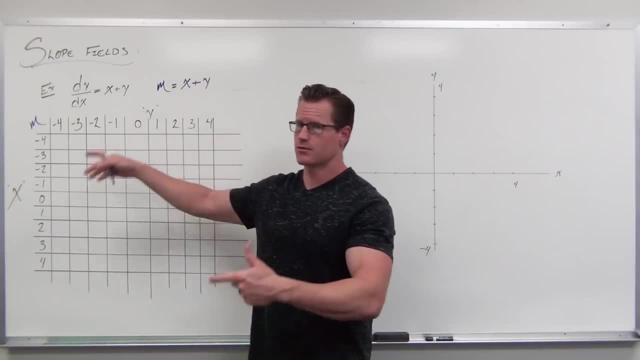 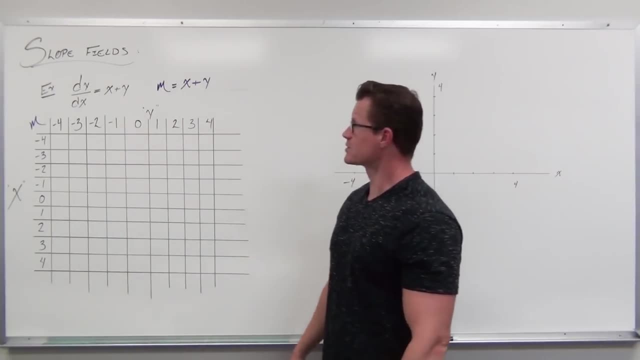 We'll talk about it in just a minute. Now you can do this however you want. I prefer to put my y values up top and my x values on the side. You can do it differently if you'd like to, But the point is try to find a pattern and then utilize that pattern. 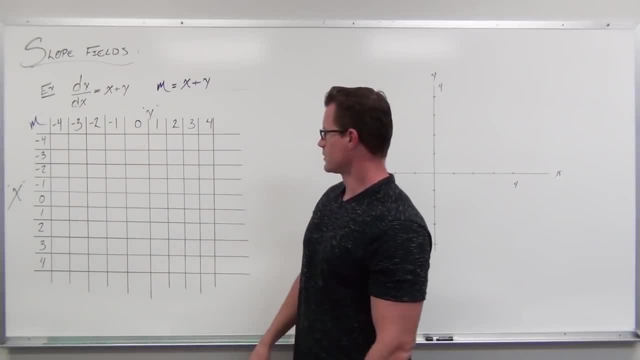 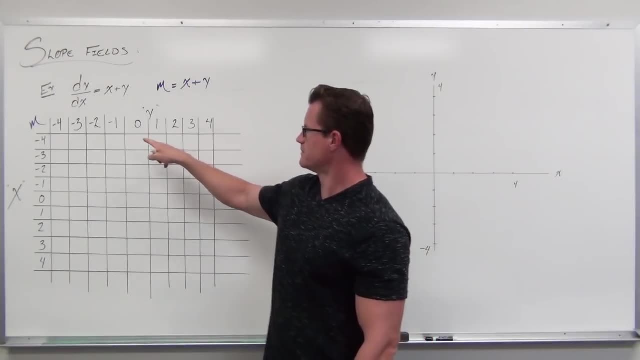 So if you want to start here, you can. I might start looking for something like: well, if I'm adding up some numbers here, I know that negative 4 plus 4 is going to give me 0.. Are you seeing that? 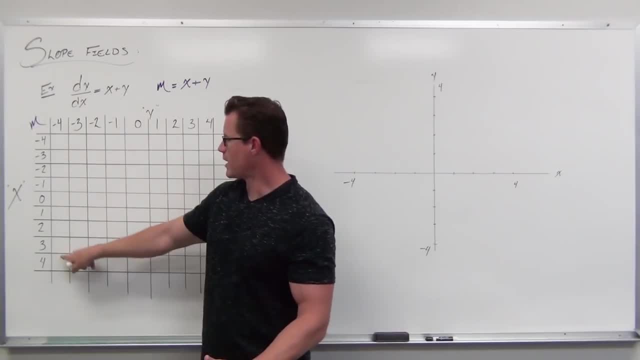 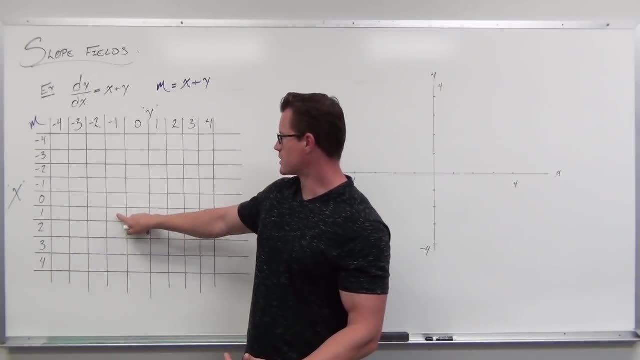 4 for my x plus negative 4 for my y is going to give me 0., But so is 3 plus negative 3 and 2 plus negative, 2 and 1 plus negative 1 and 0 plus 0 and negative, 1 plus 1 and negative 2.. 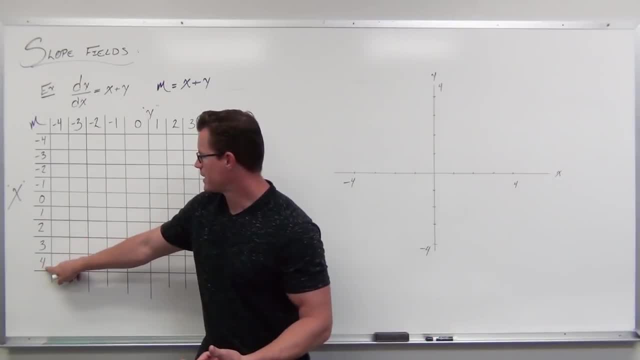 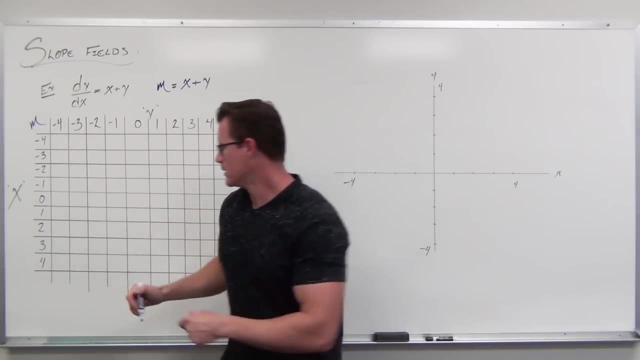 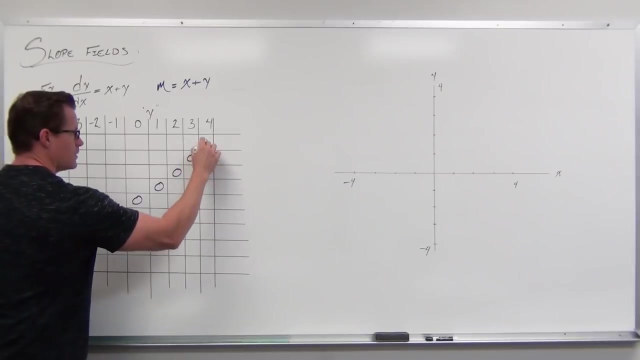 So all this diagonal is there. The x value is 4.. The y value is negative 4.. When you add them to find the slope which goes in this field, you get 0s all the way along that diagonal. You can check it if you really want to, but negative 4 plus 4 is going to give you 0. 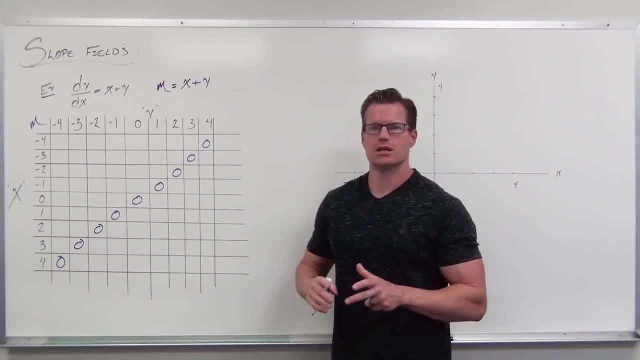 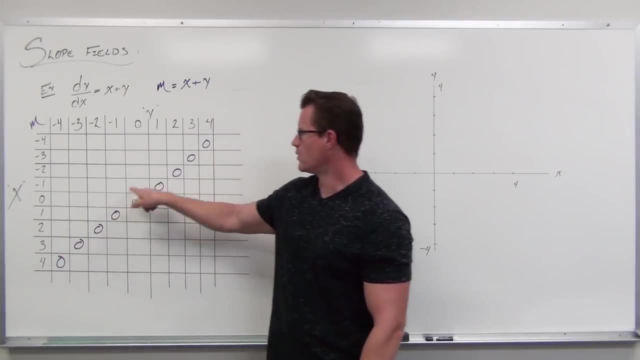 We get that the whole way. Now your pattern is going to continue diagonally for this whole rest of it. So if you find your first diagonal, all you need to do is find it. All you need to do is find one number, and all these are going to be the same. 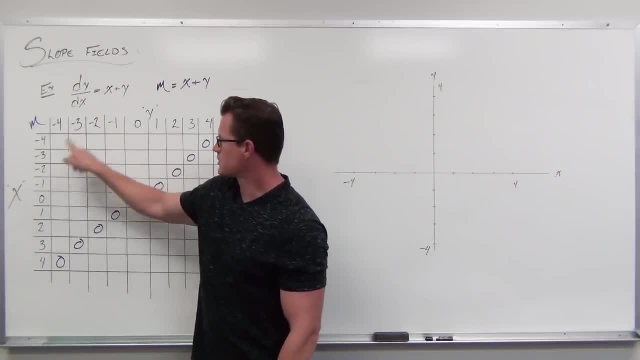 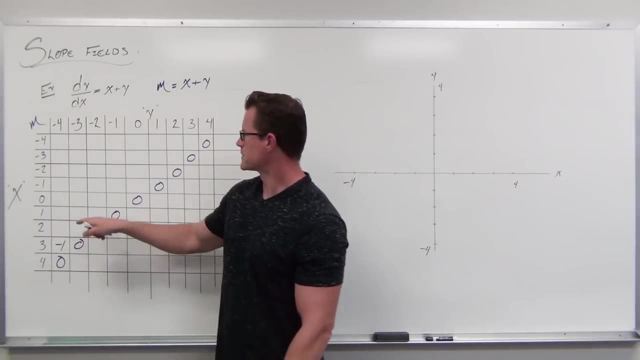 So 3 plus negative 4, x plus y, 3 plus negative 4 is negative 1.. Maybe try it for a couple of them. So for these simple ones, we get these nice diagonals. Do they all work like that? 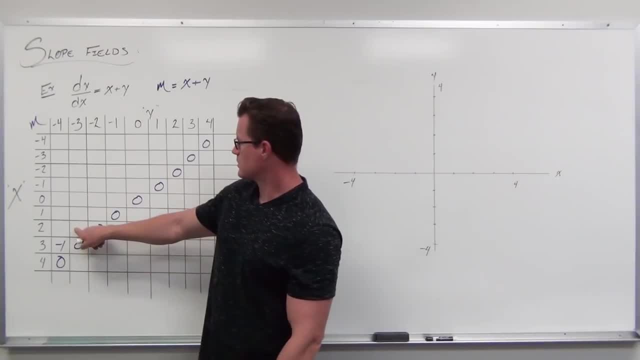 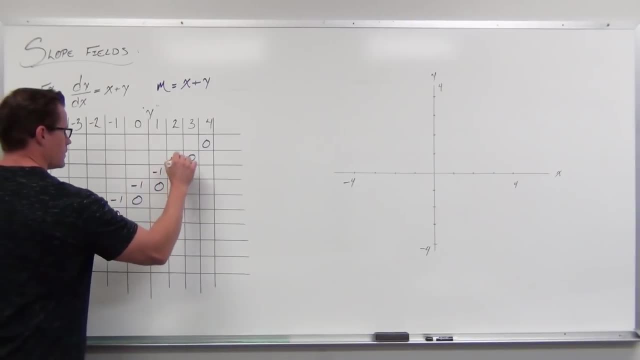 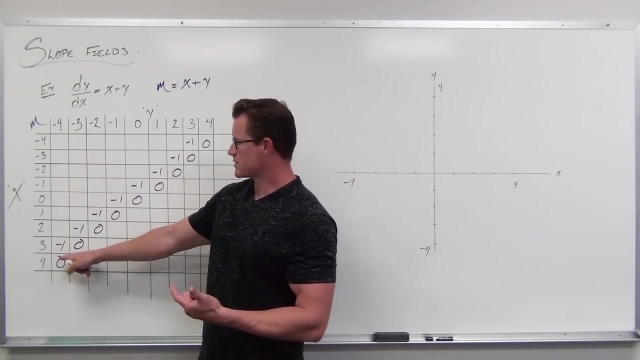 No, but a lot of them do, And so we're going to try that. So 2 plus negative 3 is negative 1.. Also, you probably could make patterns this way: So 0 and negative 1, that's probably negative 2.. 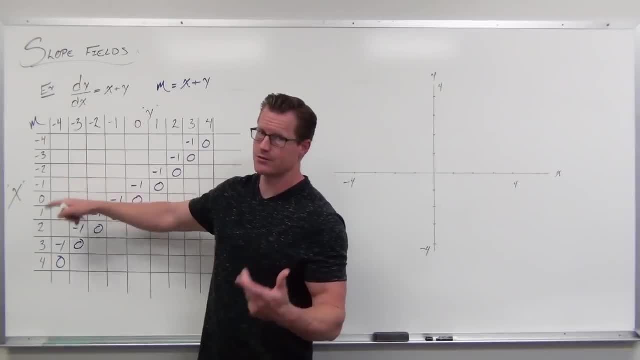 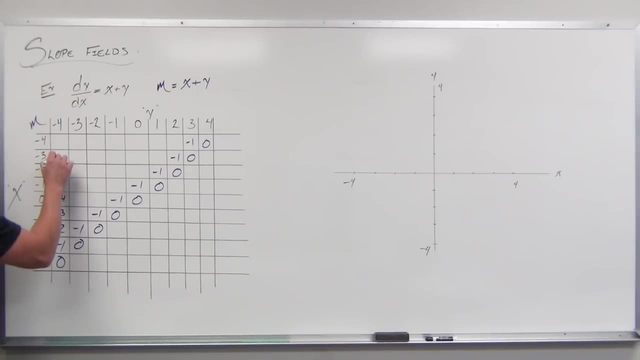 That's probably negative 3.. That's probably negative 4.. That's probably negative 5.. It works that way too, And sure enough, negative 4 plus negative 4 is negative 8.. Now we're going to continue our patterns. 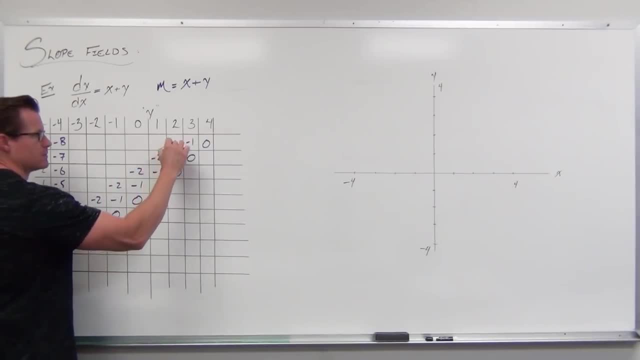 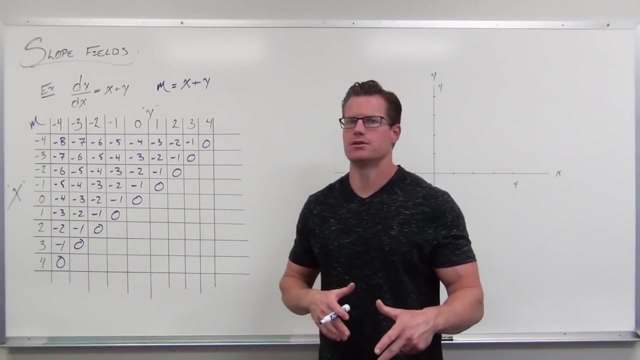 I'll use my diagonals right now, And we've already got half of our slope field done. That's pretty nice. So if you're going to have to do this by hand, most of the time you can find some nice patterns If you can't use your computer. 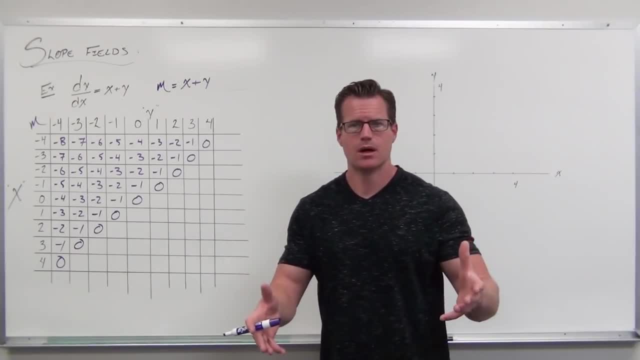 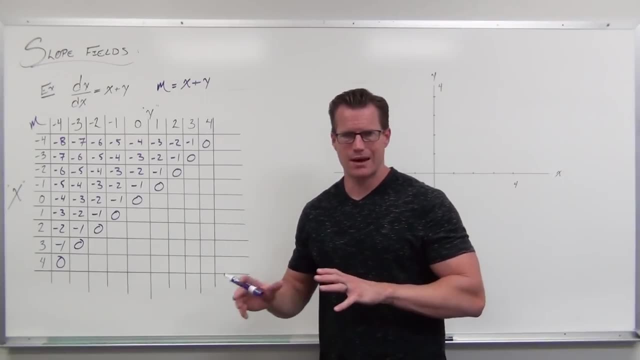 This is just to give you an idea of what a slope field is. I'm not going to explore that with you. You can use a computer or calculator to plug that in. Usually every single textbook that's out there has some sort of a graphing utility. 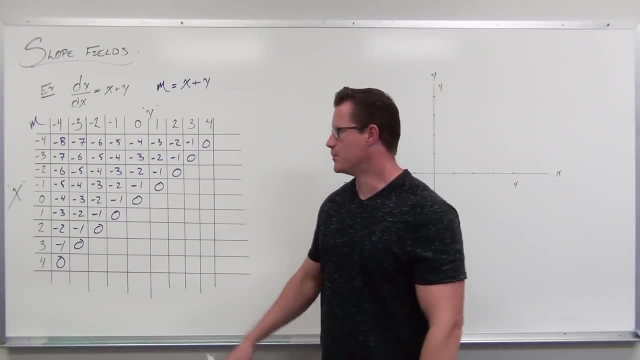 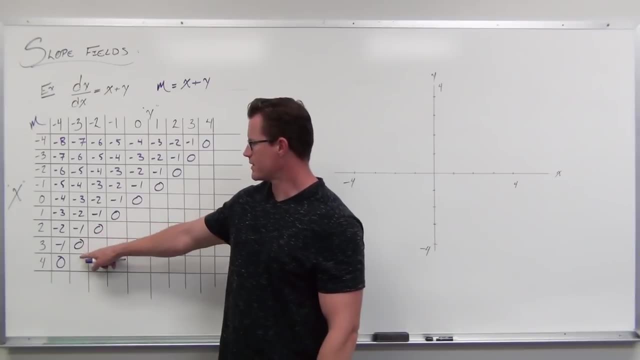 You can walk yourself through. They're not bad. Check them out for yourself. But this is just to get the idea of what a slope field does in your head. Same thing works here. So if this is negative 1, 0, that's probably 1.. 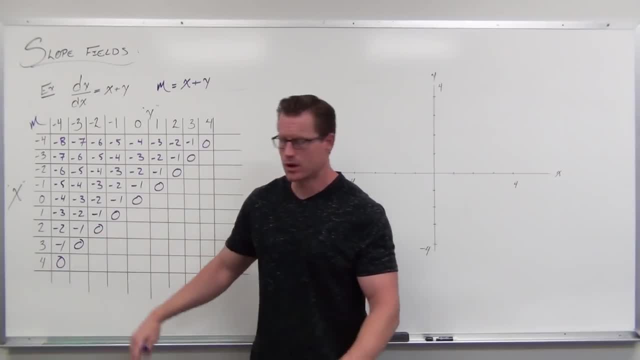 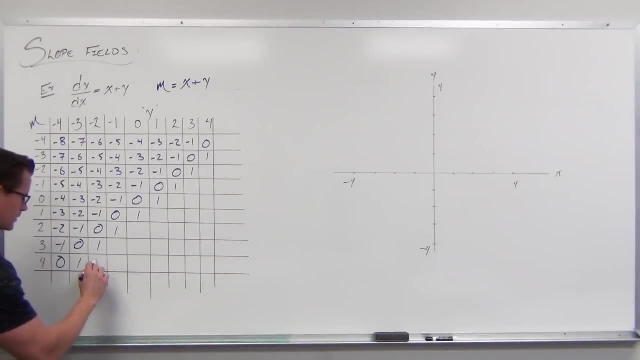 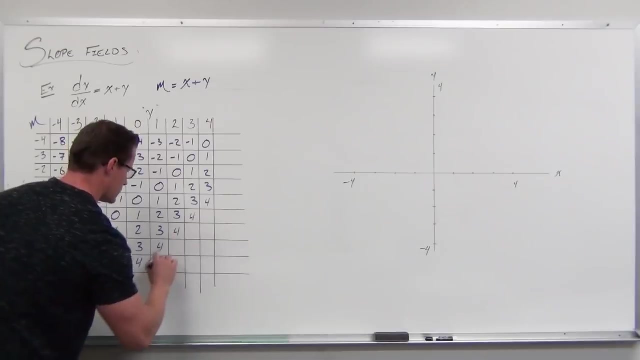 Let's just check real quick: 4 plus negative 3, that's 1.. That's probably 2.. It is So now what we've done? we've taken this thing, this differential equation, which has a first derivative in it, which means slope. 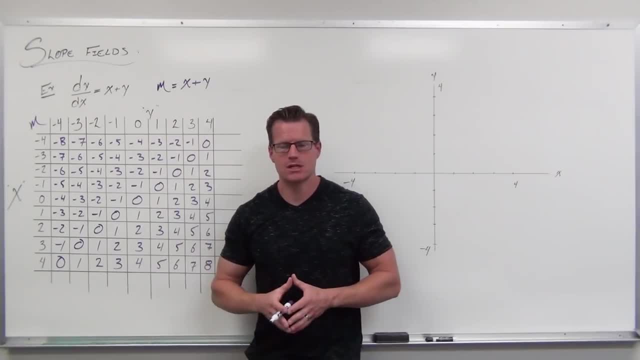 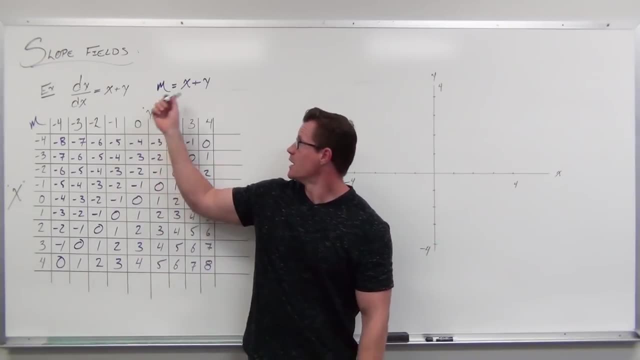 and we have a formula to find it. We just plug in every single point for this finite graph that we have. So it's limited, but you could extend it, I suppose. And we find the slope by just adding the x and the y coordinates. 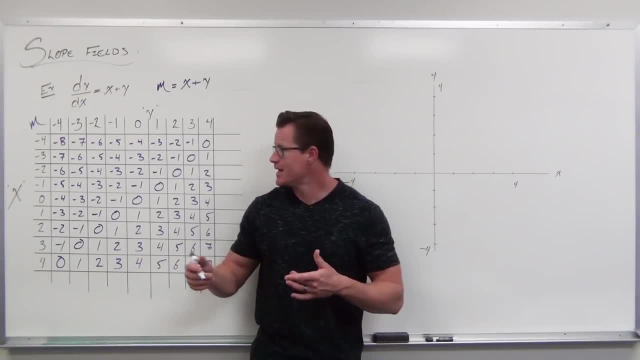 That's for this specific differential equation. Now we take all of these slopes and for, point by point, we're going to put just a little line on this graph to represent the slope. at this point It looks like a unit vector without the arrows. 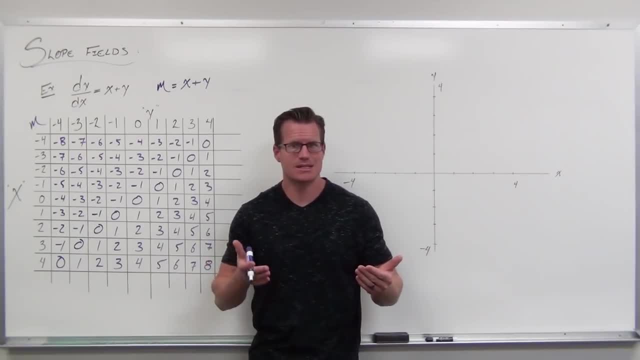 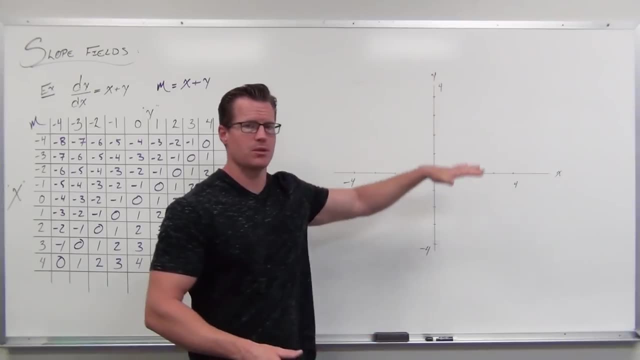 It's giving you the direction. That's what slope does. It gives you the instantaneous rate of change Or the direction that the curve is going. at that point, What that's going to do is fill up this entire x-y plane with all these sort of slopes that represent your general solution. 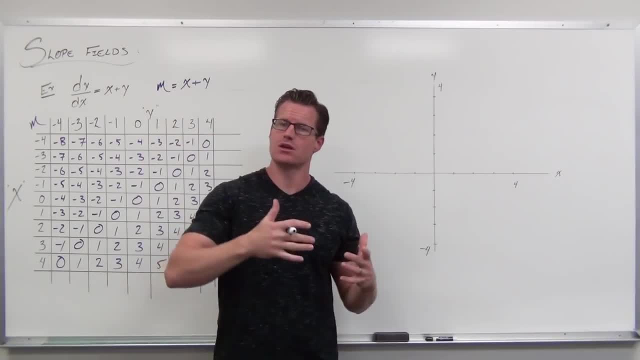 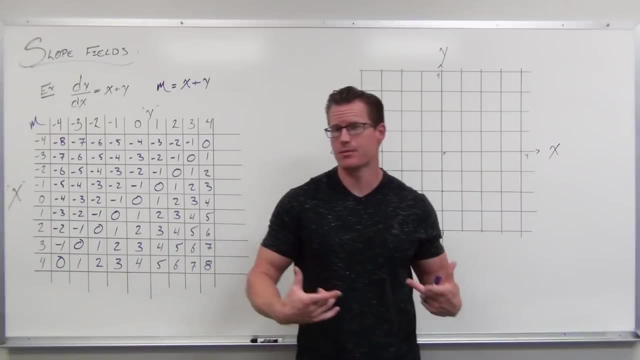 All the curves that would fit these slopes. So we'll get to that right now. Okay, so now that we have this filled out with all of our slopes at every point that we really need on the x-y plane, what we're going to do is put those little lines at every one of these points. 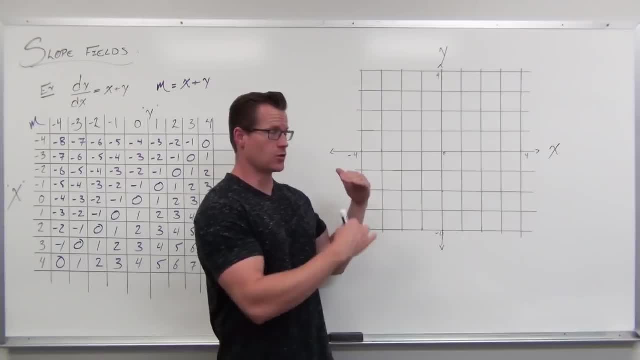 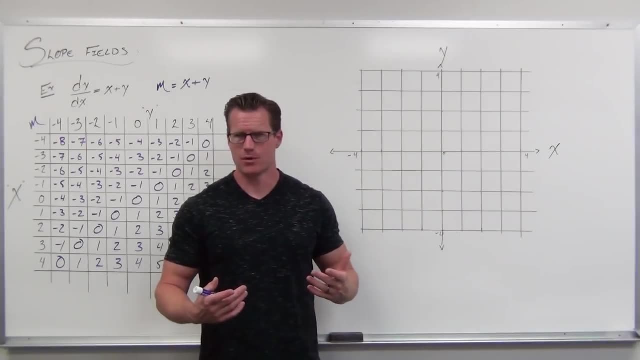 I tried to do this the first time without the grid. That's really hard. It's going to get all disorganized. So make yourself a grid, or get some grid paper, some graphing paper, That way you know at every single one of those intersections. 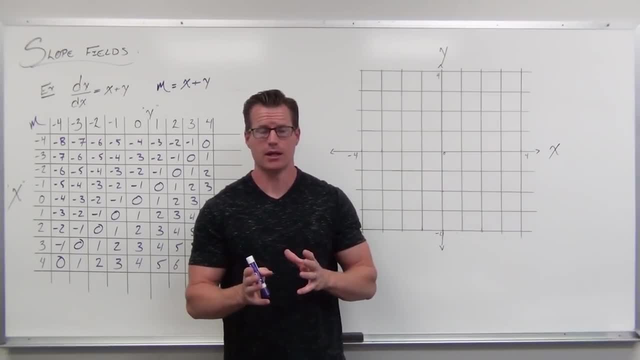 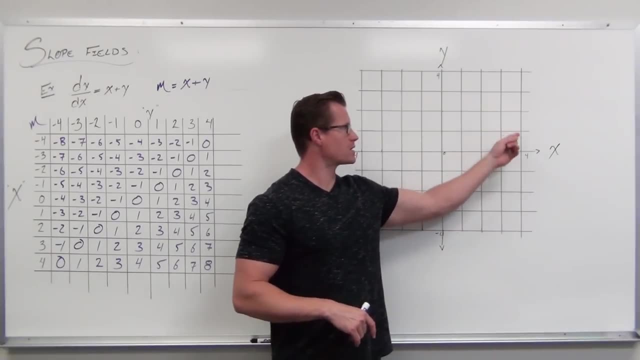 of your x and your y. that's where you're going to put your little line. So when we do this slope field, what's happening is that at every single cross section of an x and a y, we now have a corresponding slope. 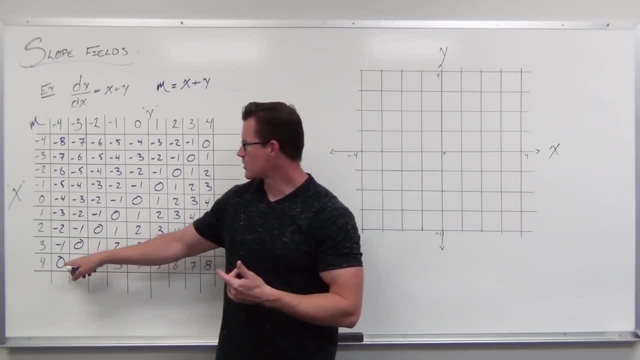 So we just have to go along. I'm going to use my diagonals. I'm going to start at 4, negative 4, and I'm going to make a diagonal. So 4, negative 4.. x equals 4 and y equals negative 4.. 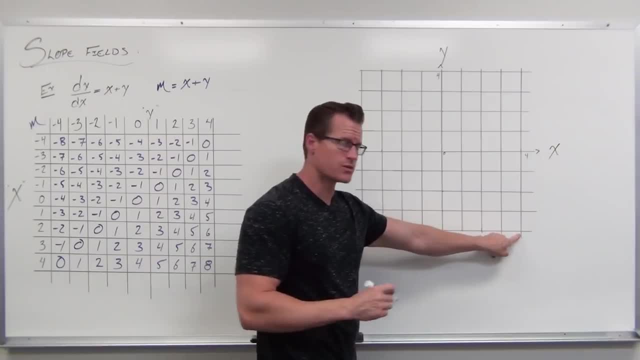 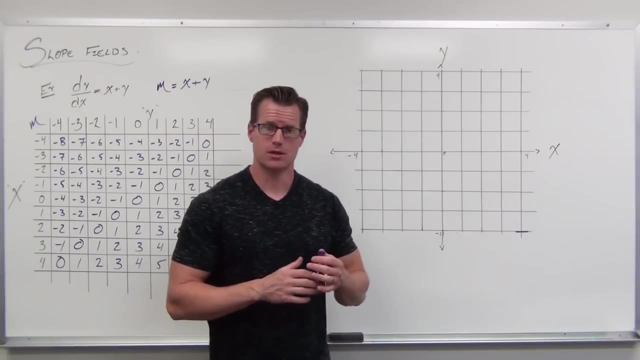 x equals 4, y equals negative 4.. I have a slope of 0. So if there's a particular solution that hits that point, it is going to have a slope of 0. at that point It's going to be flat. 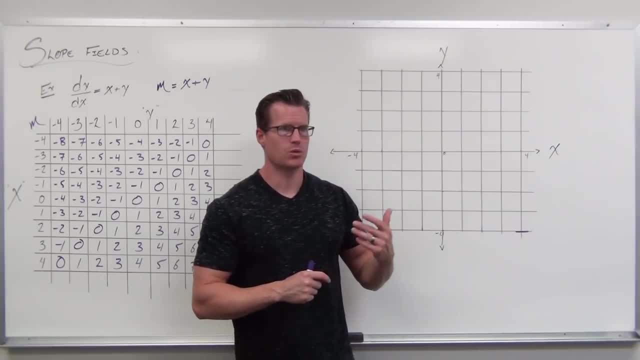 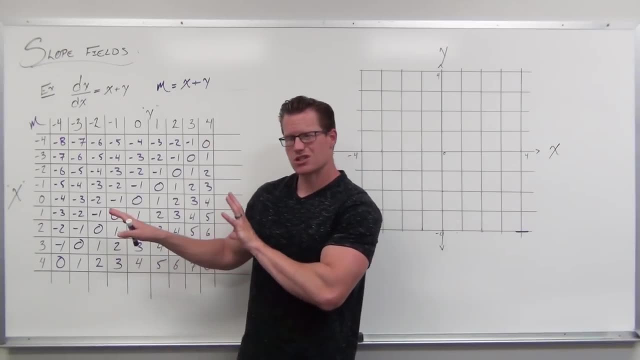 So it's probably going to be like a relatively flat slope, A relative max or a relative min is going to bounce Somehow. it's going to do that Now because you have these diagonals. just follow your pattern At 3 on the x and negative 3 on the y. 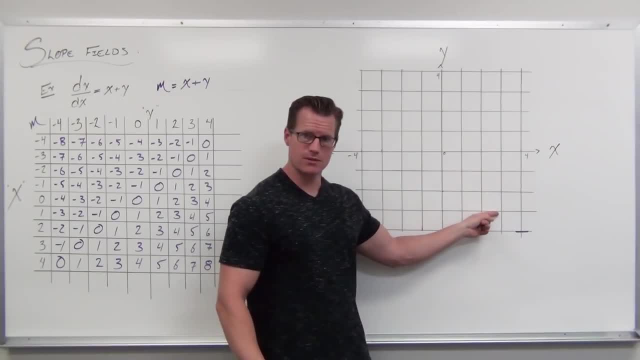 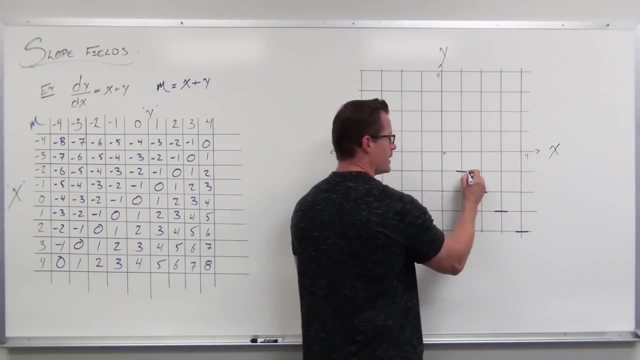 3 on the x and negative 3 on the y. we're also going to have a slope of 0. And we're going to have that at every one of these intersections. Hopefully you can verify by looking here that. yeah, you know what. 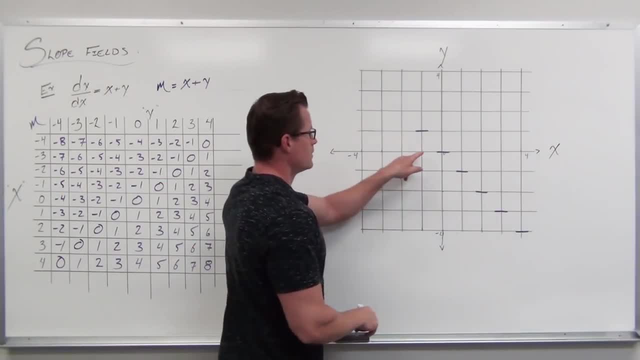 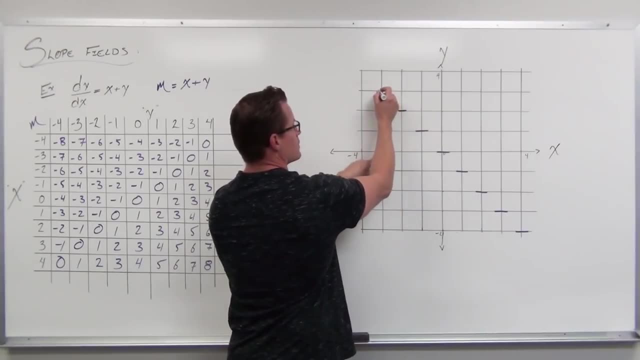 At negative 1 on the x and 1 on the y. negative 1 on the x and 1 on the y. I have a slope of 0. And at negative 2, 2,, negative 3, 3, and negative 4, 4,. 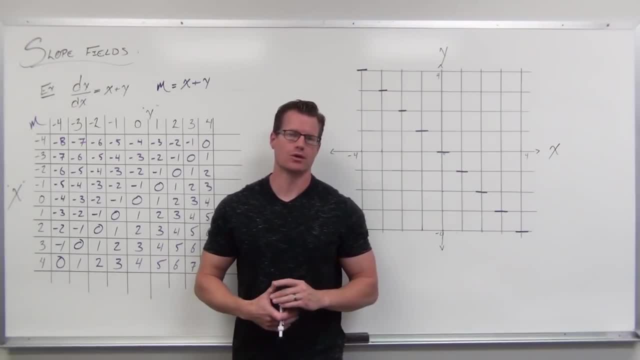 those all have a slope of 0.. That's how a slope field works And we're going to take some time and just fill this out. Maybe you can do it as I'm doing it If you've drawn this. If not, just follow me along. 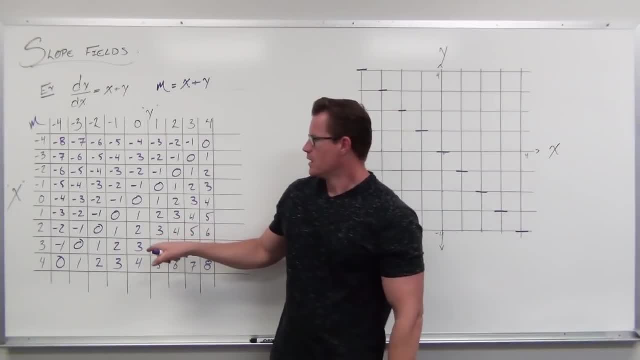 That's okay. I have another one in just a minute that you can do on your own if you'd like. So be careful. It's kind of easy to get these confused, especially confusing your x with your y, So I pause for just a minute. every time I start a new diagonal. 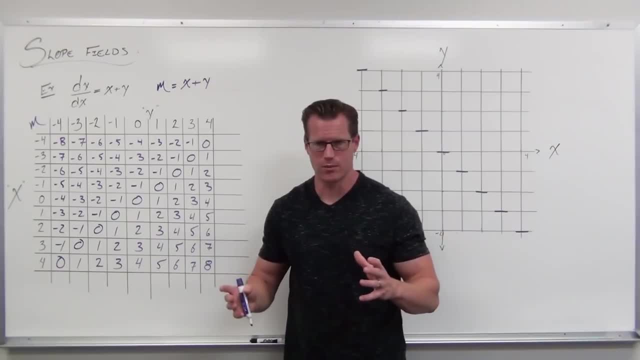 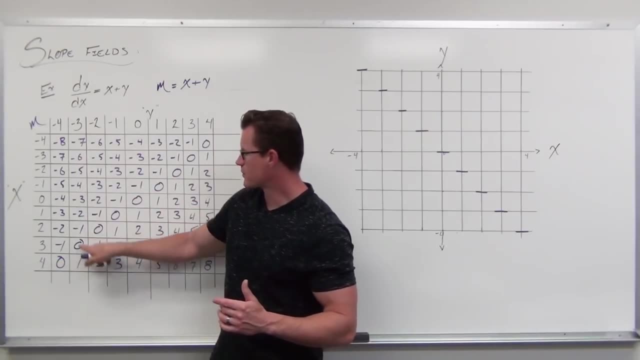 And I make absolutely sure that I have the right starting slope for whatever point I'm on. So I'm going to go and do 4 on the x, negative 3 on the y. I'm going to put a positive slope of 1.. 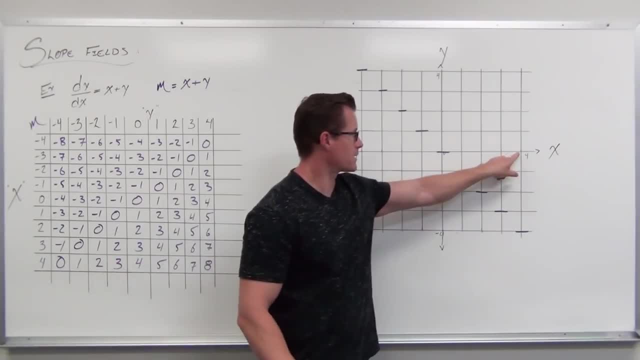 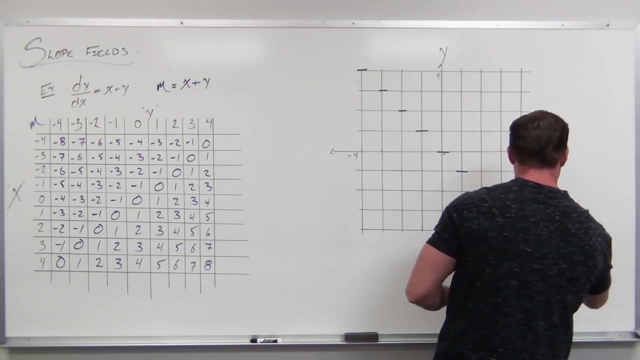 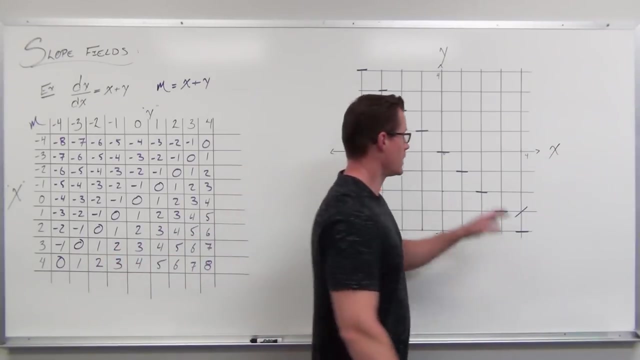 So 4 on the x negative, 3 on the y, 4 on the x negative, 3 on the y, And that's got to have a slope of 1.. Now I'm going to see how that pattern works. So the next one: 3 on the x negative, 2 on the y. 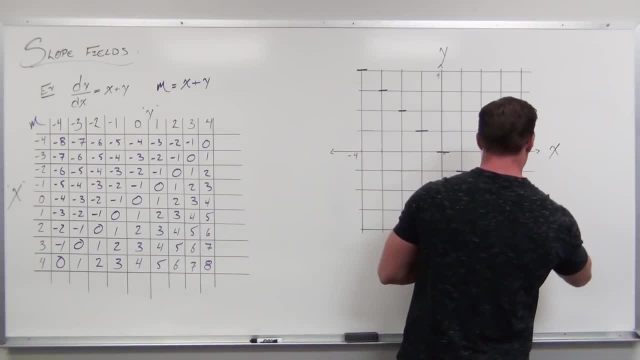 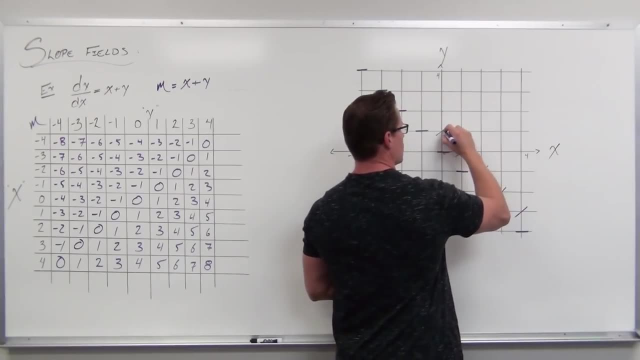 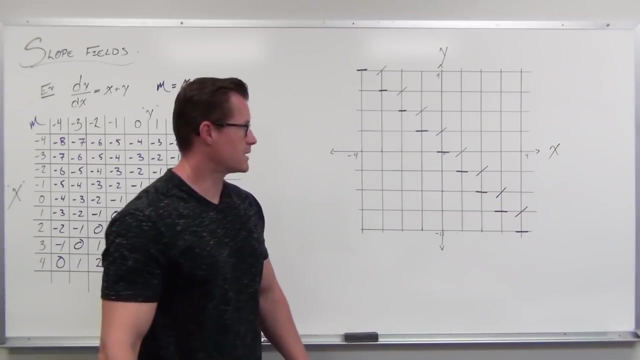 3 on the x, negative 2 on the y, And I'm going to try to give that the same slope all the way up, And drawing that grid makes it just infinitely easier. Not infinitely, but a lot easier. OK, let's keep on going. 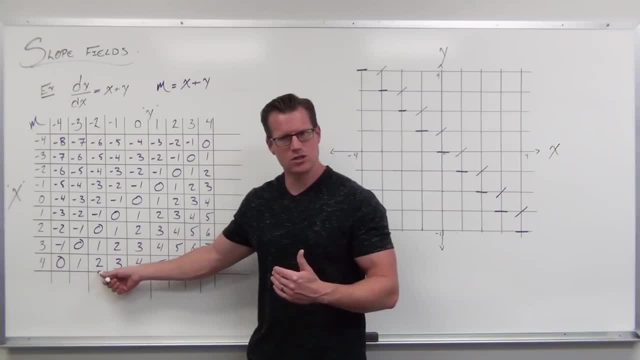 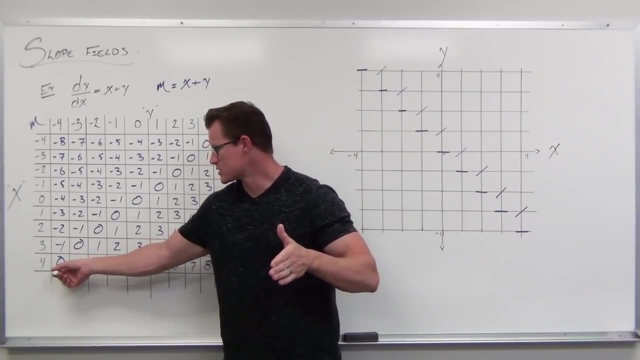 Also we can use this pattern down here. So as we're going on the x equals 4 vertical line. so going up the y's, our slope goes from 0 to 1 to 2 to 3, to 4, to 5, to 6, to 7 to 8.. 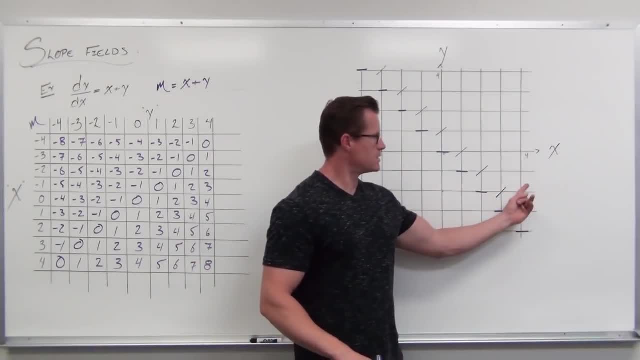 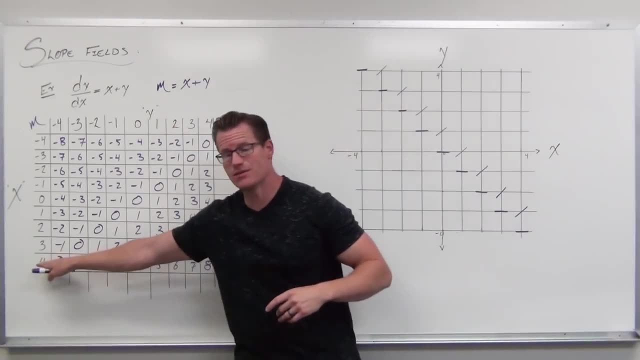 Here's what that means. This is a slope of 0, 1,, 2,, 3,, 4,, 5,, 6, 7, 8.. It's going to be really steep. So as we climb along our y for a given x value. 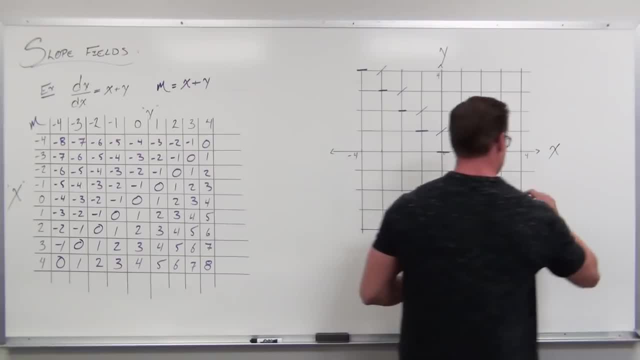 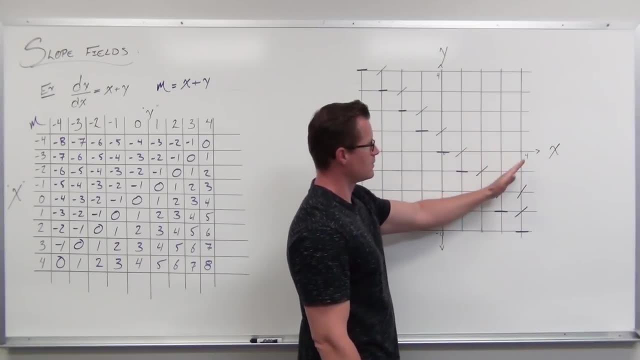 our slope is going to be 0.. Our slope is increasing, So you could do that too. There's about a slope of 2.. So I'm going to continue that diagonal. I'd have a slope of 3,, 4,, 5,, 6,, 7, and 8.. 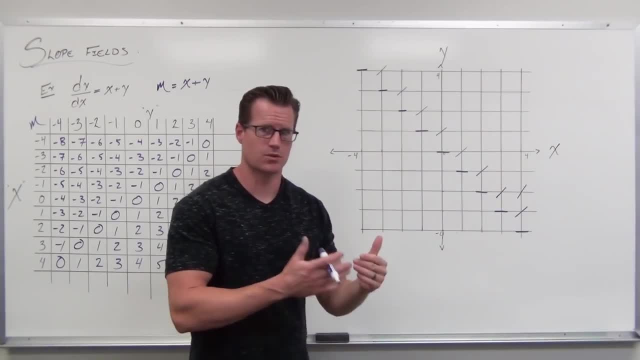 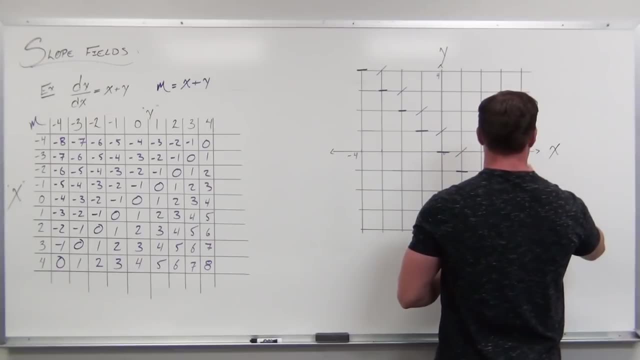 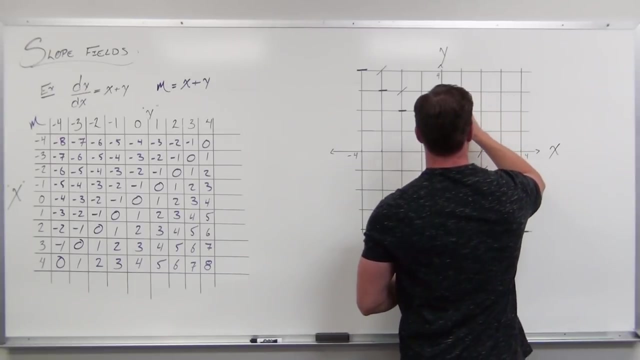 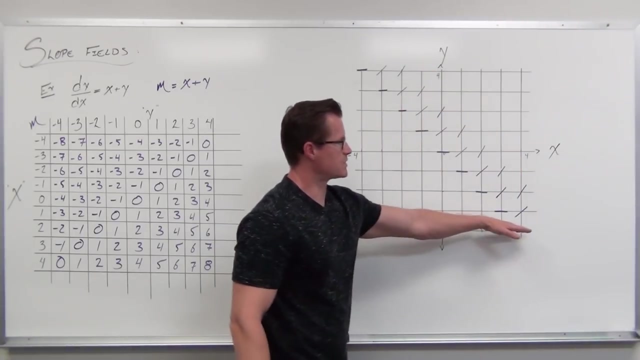 You're approximating here, So your slopes are going to get really, really steep by the end of it. So at 0,, 1, I followed it. 2, I followed it. I know this is going to be 3.. 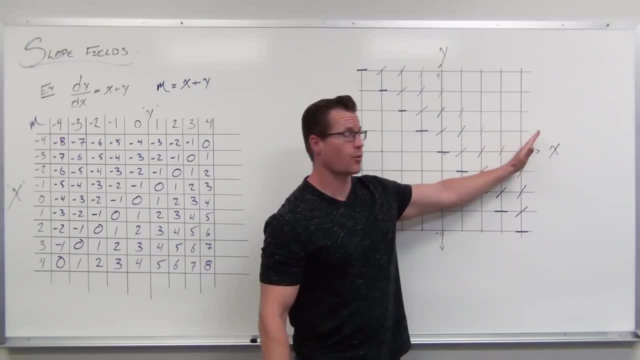 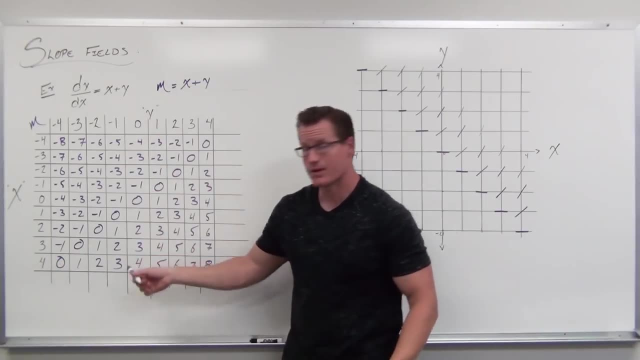 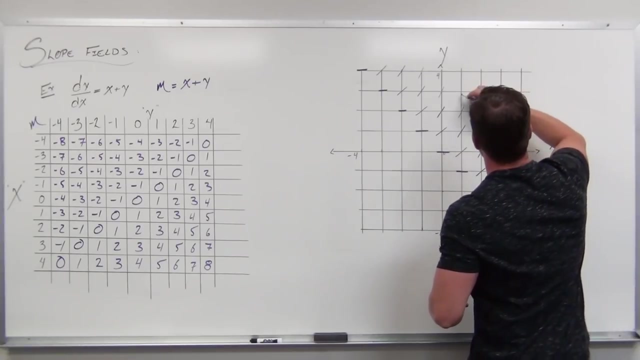 0, 1,, 2,, 3.. It's pretty close. Here's going to be 4.. So at 4 on the x and 0 on the y, I'd better have a slope of 4.. 4 on the x, 0 on the y, I've got a slope of 4.. 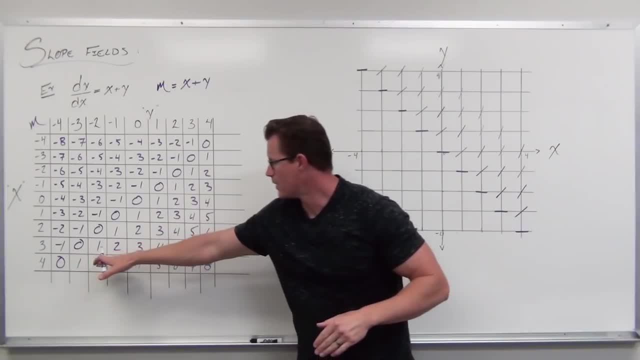 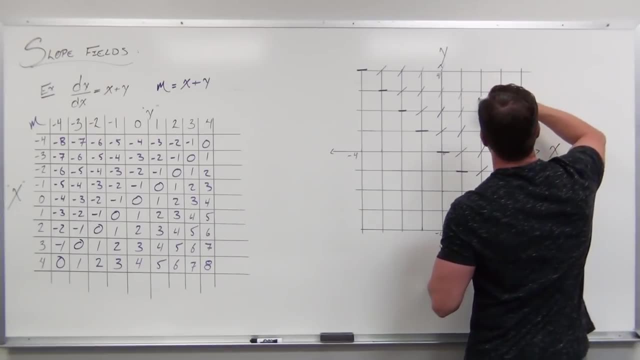 Next I should have a slope of 5.. I'm going up on that x value and my slope is increasing: 4., 4., 4., 4., 4., 4., 4., Then 6.. 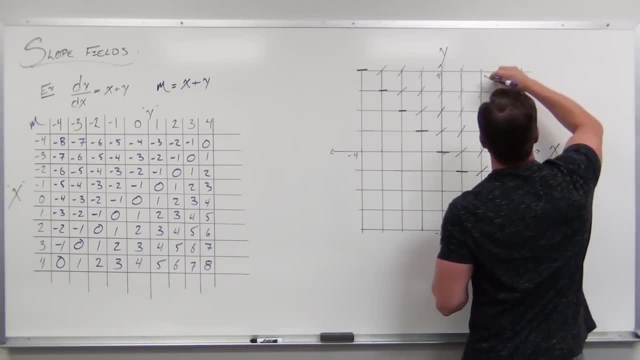 Then 7. Then 8.. My weight's getting higher And I've doubled, So here's what this is looking like, And what this means is that every single one of our curves that fit on here has a slope of 4.. 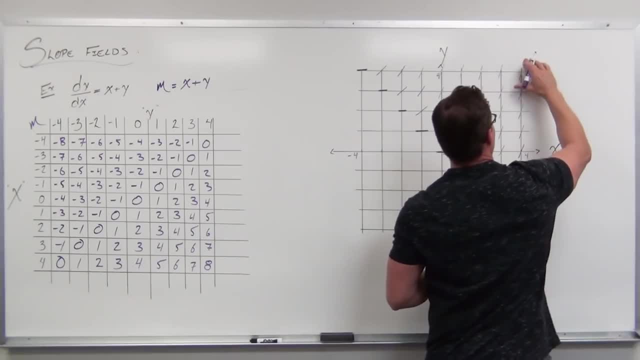 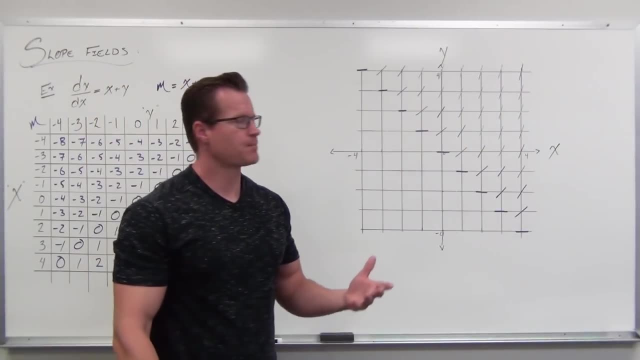 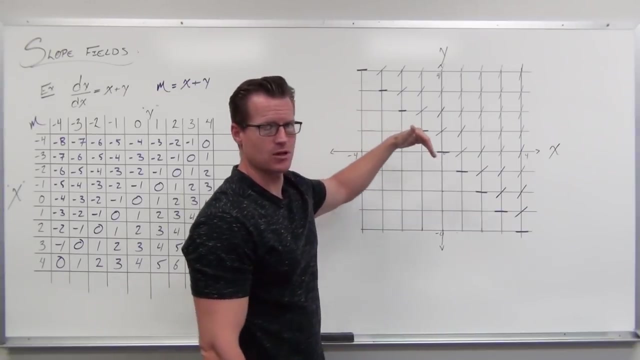 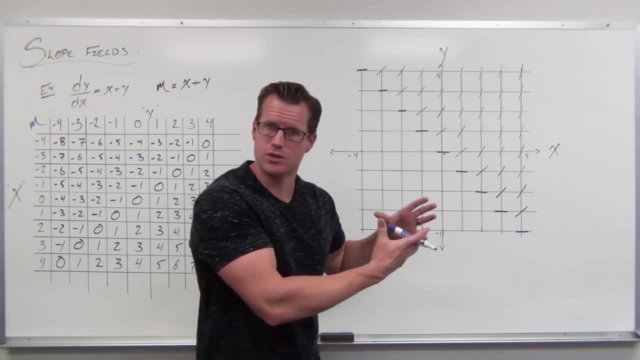 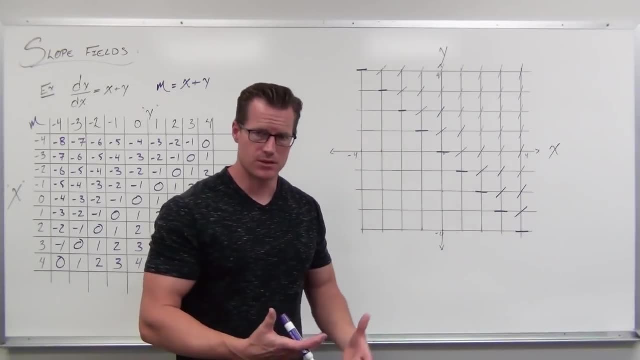 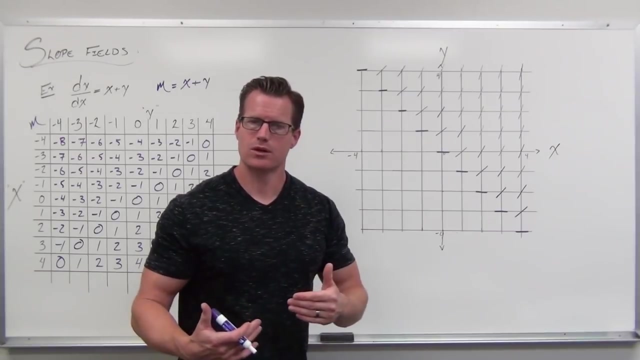 An infinite many. That's why this represents a general solution. So all of the solutions that we could possibly have would have to fit on this plane and have these slopes at their specific points. That's what I was saying earlier, that if you want to find a particular solution, one curve. 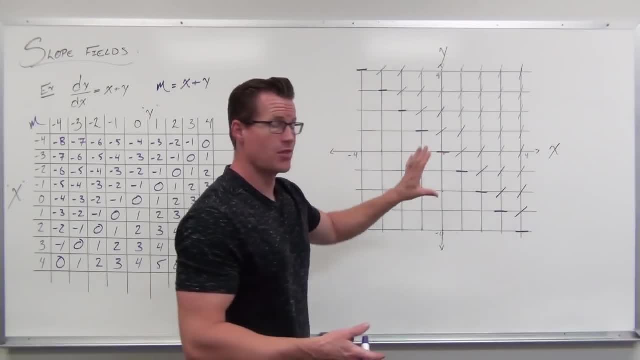 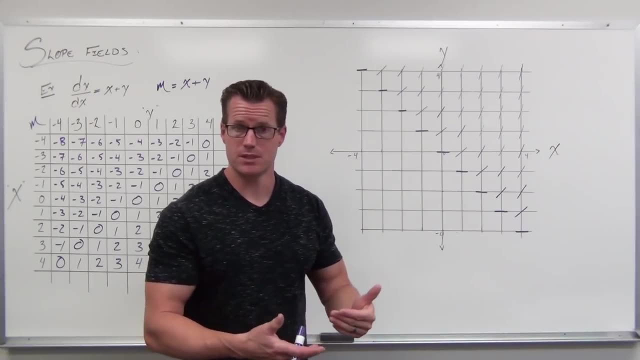 you need to start with a point. So we fill this out and then I'm going to give you a point. Let me finish the rest of this and then we'll go through and I'll give you an initial condition to find a particular solution. So let's finish the rest of our pattern. At 3, on the x and negative. 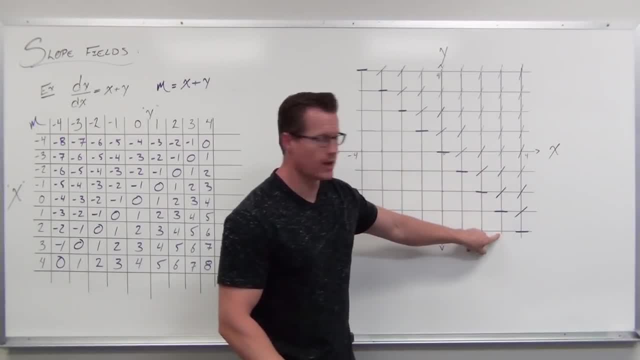 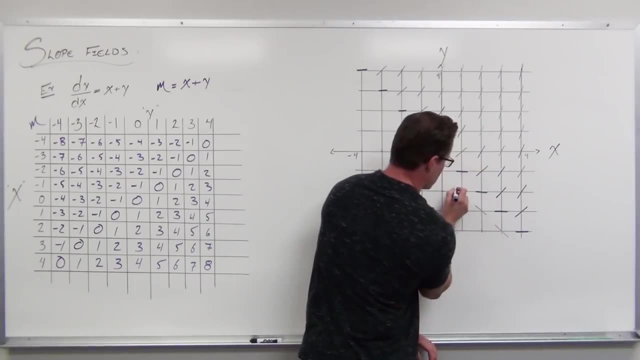 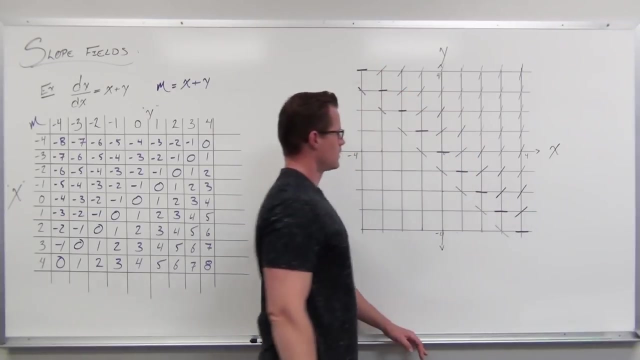 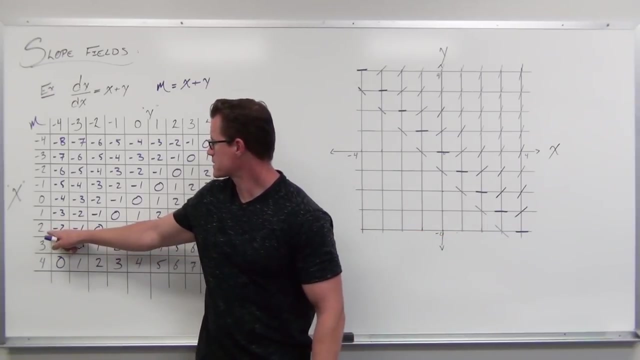 4 on the y, 3 on the x, negative 4 on the y. I need to have a slope of negative 1. At 2 on the x and negative 4 on the y. so 2 on the x and negative 4 on the y. I need a slope of. 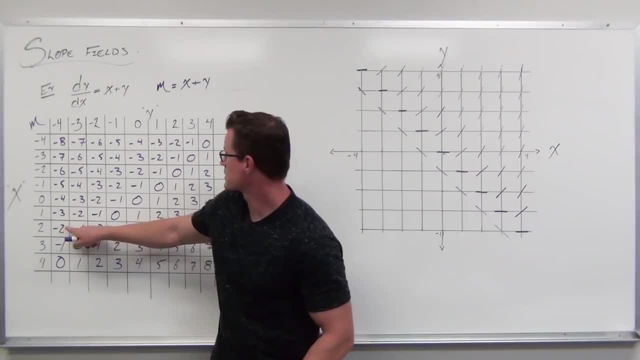 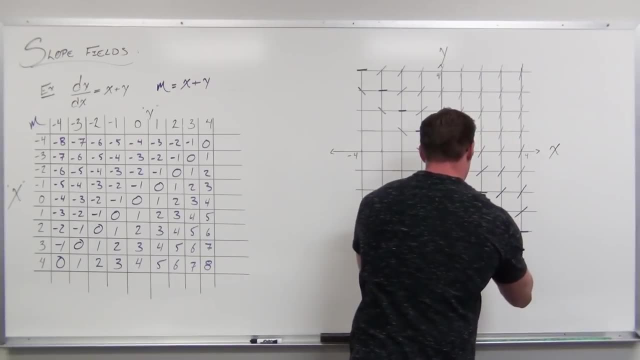 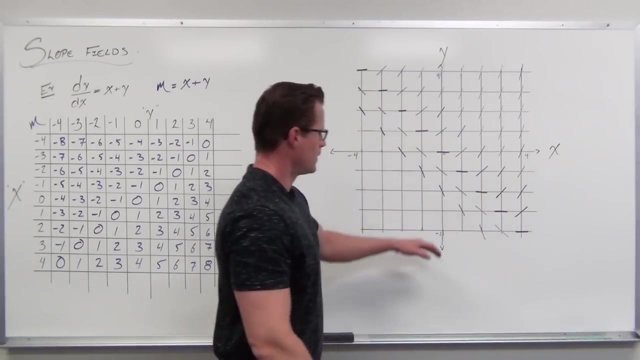 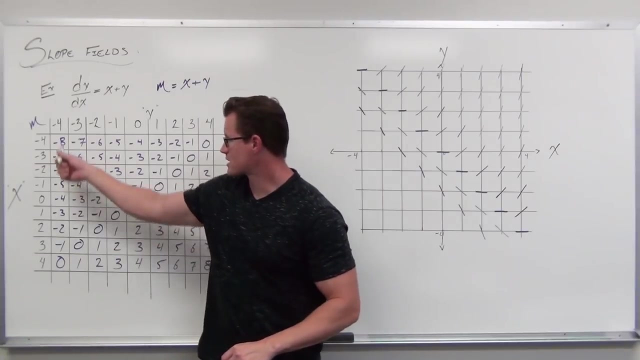 negative 2.. Let me make sure of that. 2 on the x negative 4.. So 2 on the x negative, 4 on the y slope of negative 2.. Then negative 3,, negative 4,, negative 5, negative 6,, negative 7, and negative 8,, just like we have. 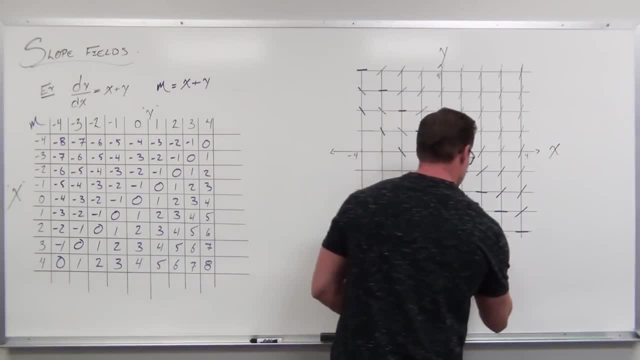 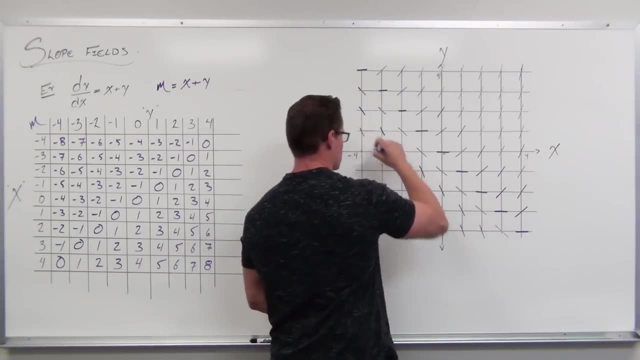 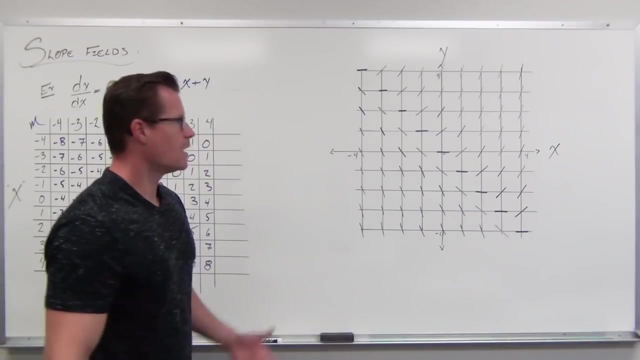 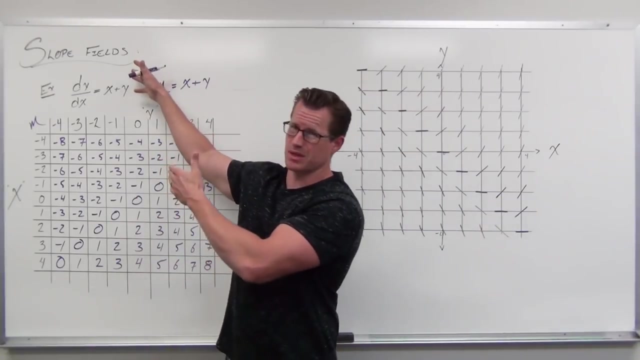 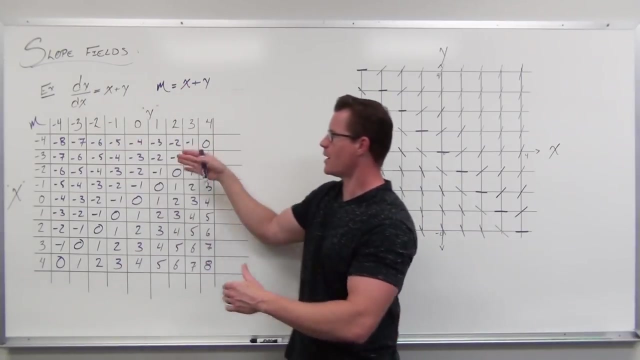 shown here About like that, and we're approaching it. I'm going fairly quickly, So let me recap it for you just a bit. Some things. we can't solve This we can probably with another technique, But we can find the slope at every point. That's what a slope field does. It says all of our x's, all of our y's. 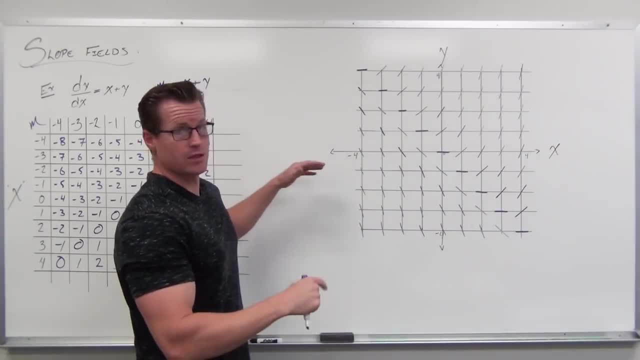 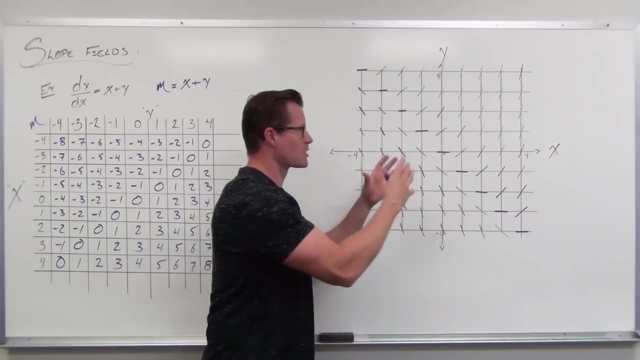 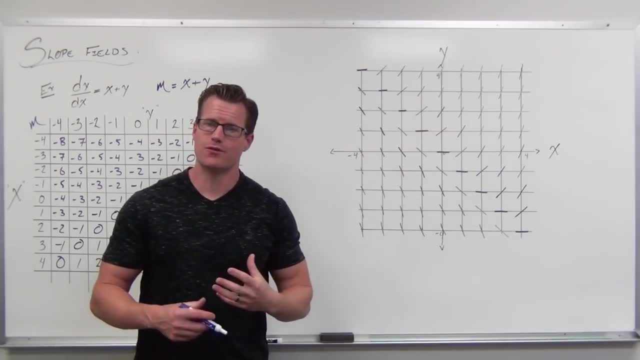 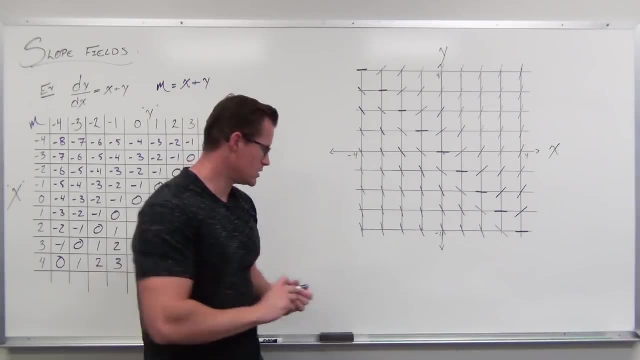 And this is the way that they would look. So to find a particular solution, well, you need to have a point. So let me show you a couple things that we can do If we had a point like 0, 0, say, 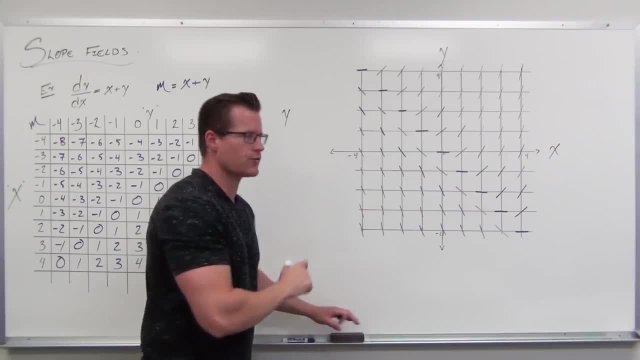 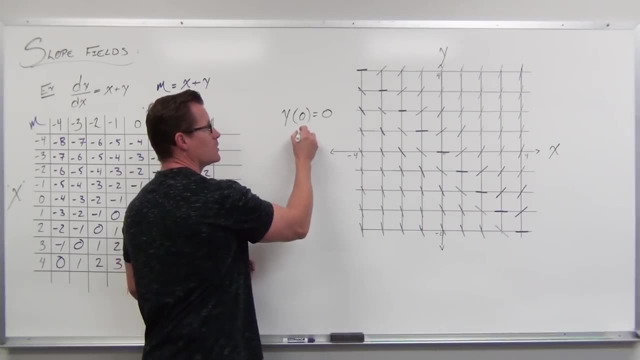 that we wanted to have the particular solution, one curve that had an initial condition of y of 0 equals 0. That would go through the point: 0 for x, 0 for y. That's right here. So we're going to. 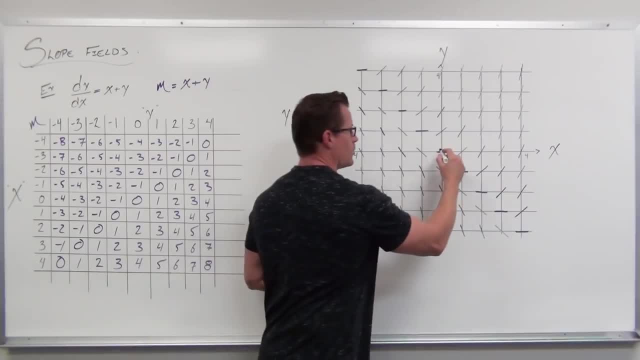 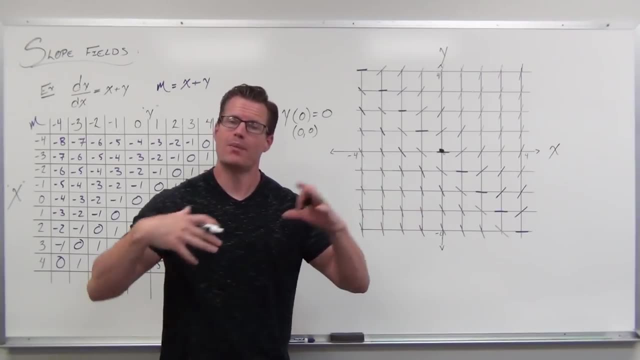 have a point. So if we're going to have to go through that point, remember what I said about every single point along this curve would have to have these slopes. Well, we're backtracking. now We're saying: what if I need a curve that goes to that point? Well, it's going to still have to. 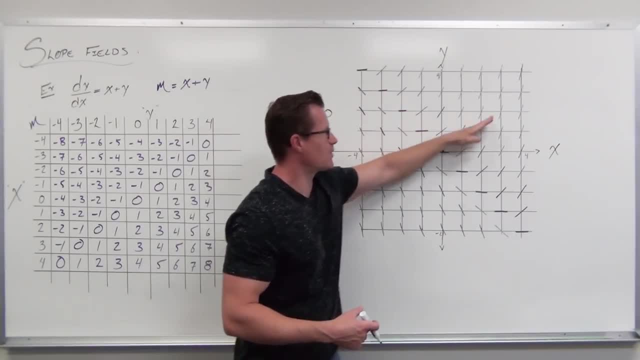 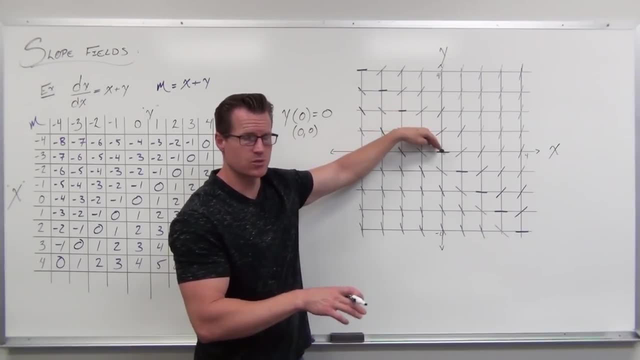 fit this. Look at how this would have to fit along these slopes. So if I'm going through that point, yeah, right here we're going to have a change from decreasing to increasing. We're going to have a local minimum for this particular curve. So we're going to have a change from decreasing to 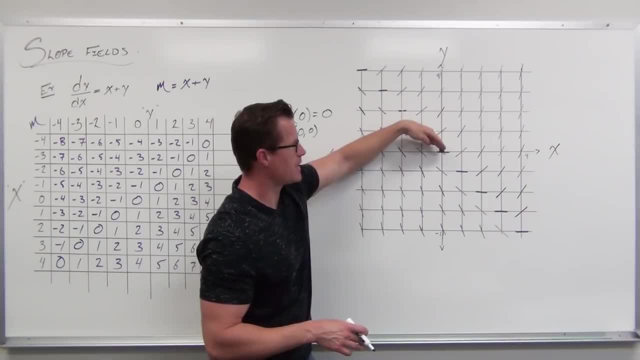 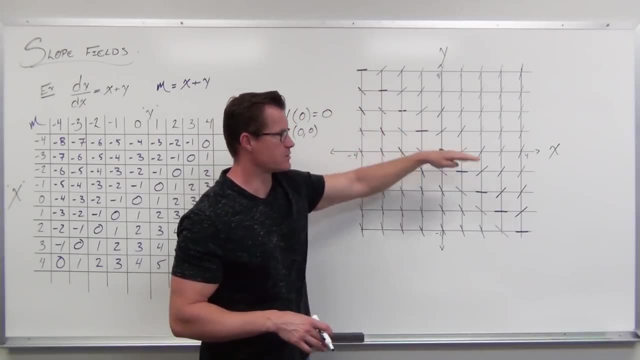 increasing. So right at that point we know that after that, all my slopes are climbing. They're all positive. They're all climbing Before that. all my slopes are negative. They're all falling as we go from left to right. So this has to really be approximated by something that goes along. 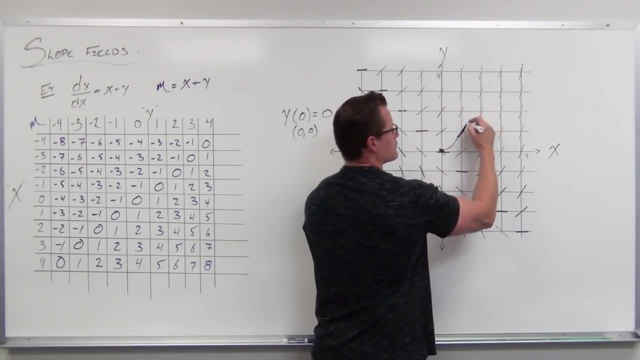 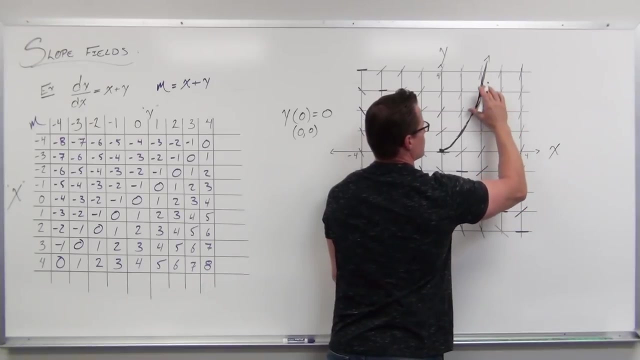 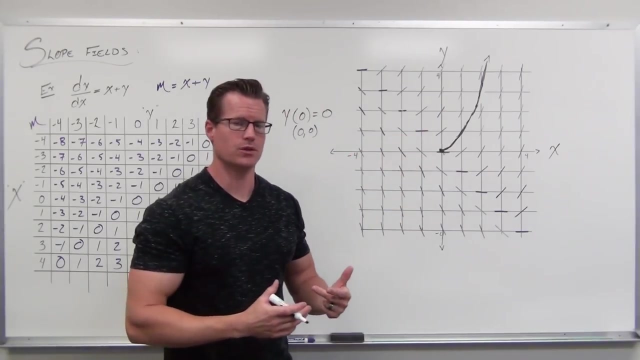 increases. Look how this is going to have. this slope here goes further. It's going to have this slope. It's going to end with a fairly steep slope That has to look something like that to fit that slope field. So once we are given a specific point, 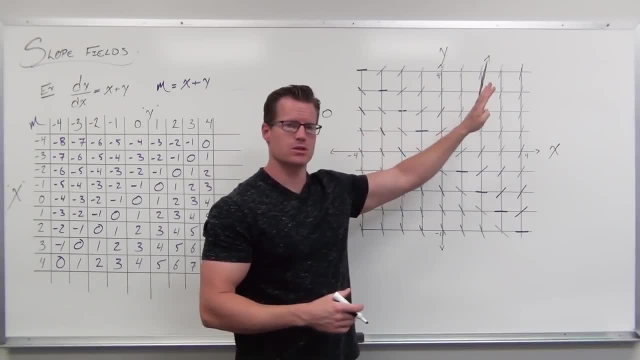 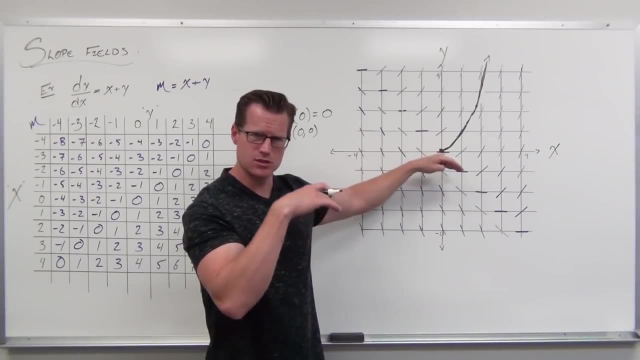 in initial condition. the rest of this flows along with our slope field. Now, before that, I know that that slope is zero. It's going to dictate that we have this change from decreasing to increasing. And look at this line. This line is going to be the same. It's going to be the same. 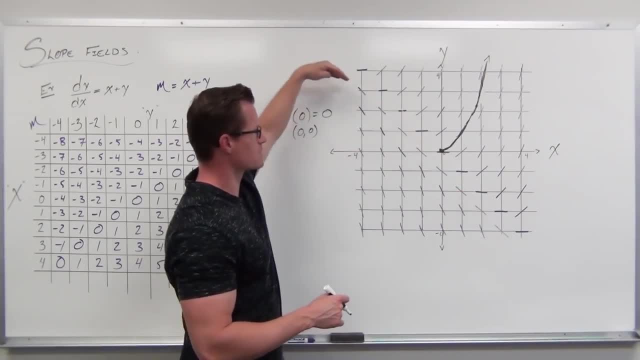 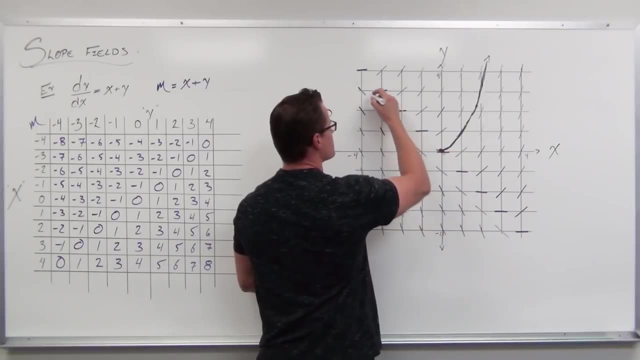 line. It's all negative one right here. This negative one slope says: hey, you've got to follow that. It's like an asymptote. So before that, we're going to have to somehow fit this And we probably look something like that. 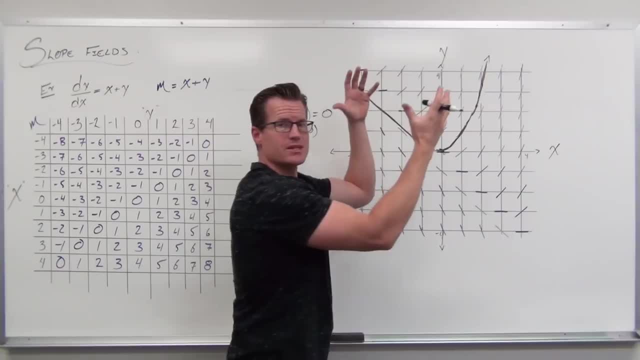 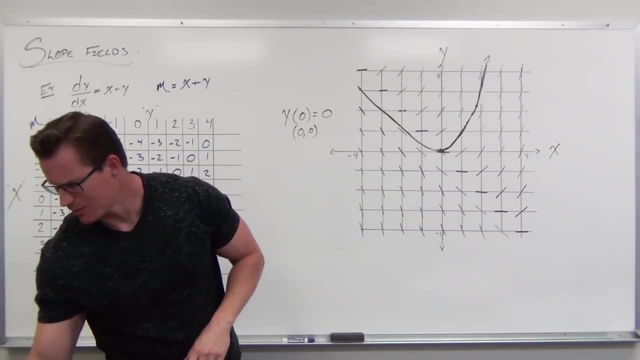 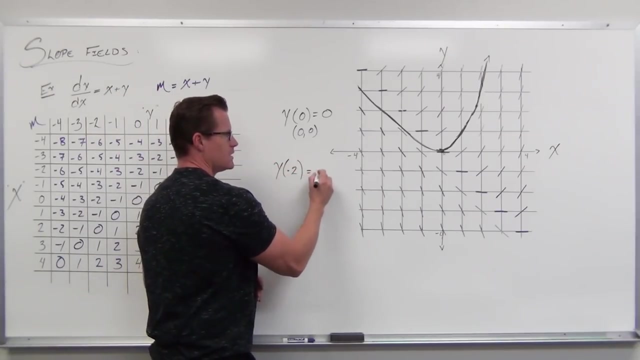 So general solution, that's the whole thing. This represents all the slope, So we're going to have to somehow fit this. All possible solutions, particular solution: you just need a point And then follow your slope field. Let's try a couple more. How about negative 2, 2?? So y of negative 2 equals negative 2.. That 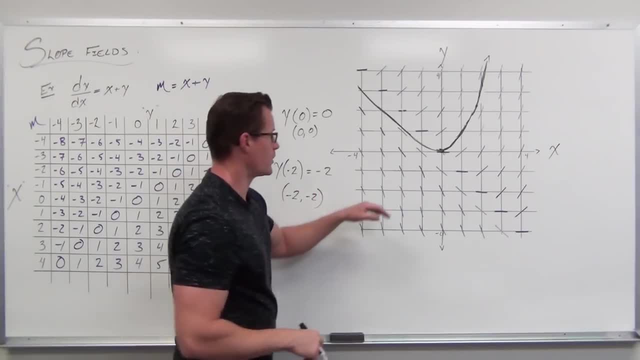 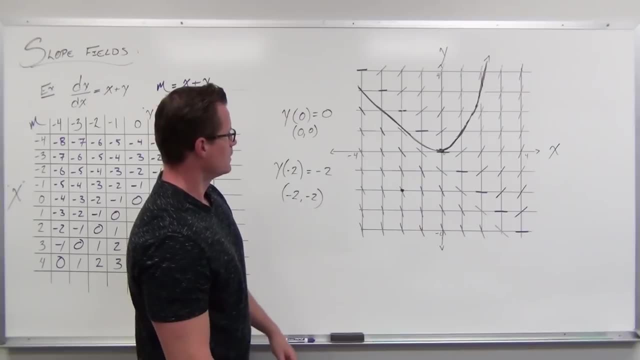 gives us a point: negative 2, comma, negative 2.. So let's go to that. Let's go to that point. Negative 2,, negative 2, that's right here. Now we're not going to be hitting this asymptote, because look how our slopes go. 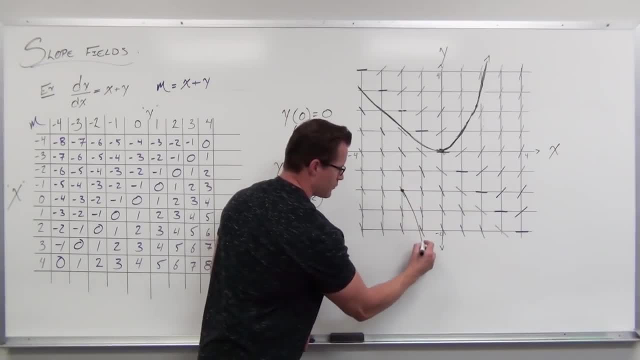 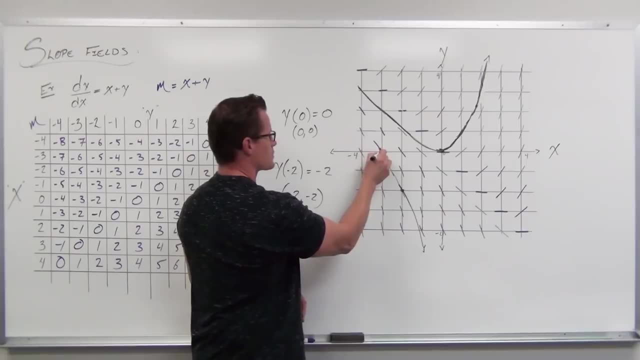 I know that afterwards I'm getting more and more negative with my slopes. I have to look something like that Before. I'm just going to follow this up. I'm going to follow my slopes. I'm just going to make sure that I'm hitting those slopes at the right slope for wherever I'm. 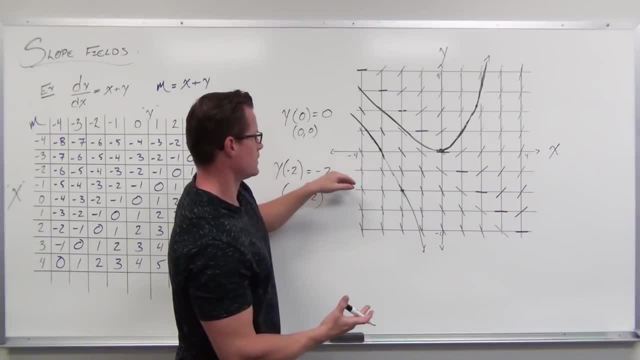 falling on my slope field. So this was, let's see, a slope of negative 1, negative 2, negative 3, negative 4.. So this would be negative 1, negative 2.. So a slope between negative 2 and negative 3. right there, That's about how that particular solution. 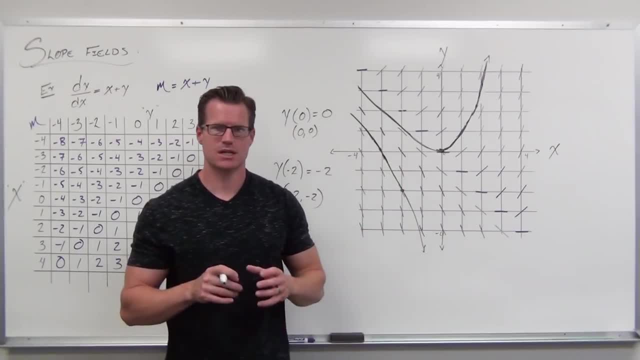 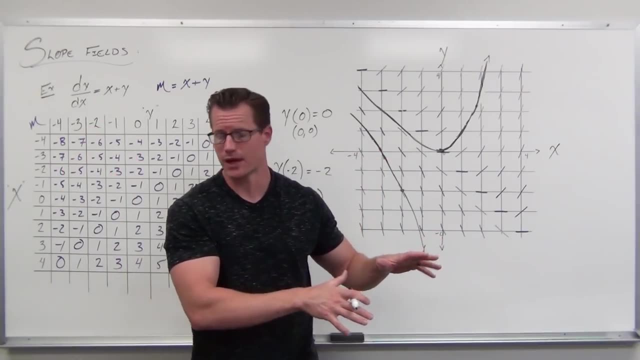 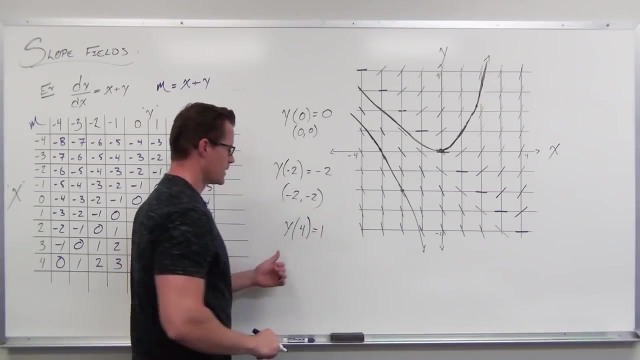 will work. I hope this is making sense to you. I hope you're seeing the idea that the general solution has all these different slopes For a particular. you need a point and just follow the slopes before and after that. Let's do one more: Y of 4 equals 1.. So when we go to this point, 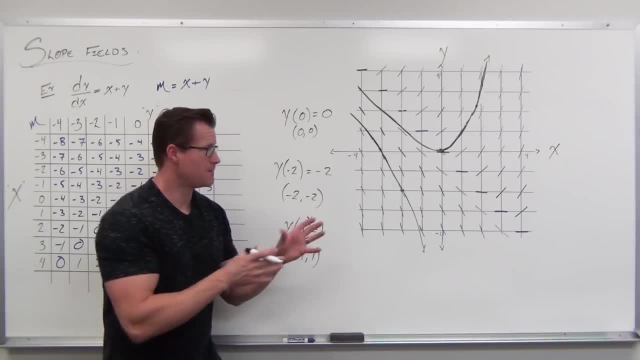 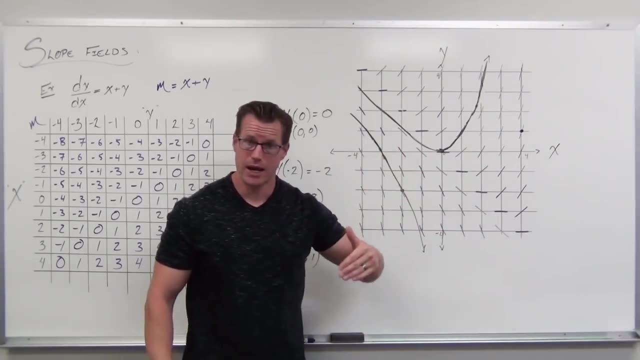 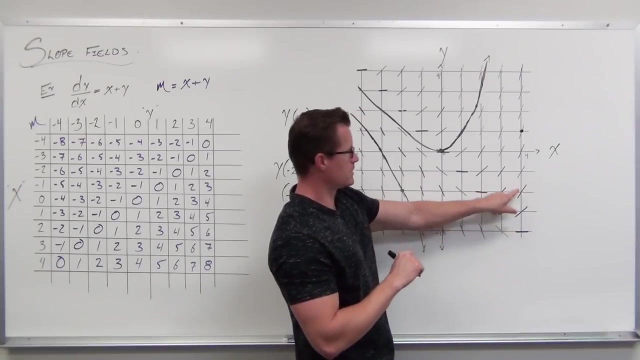 4 comma 1,. all it's saying is: make sure that when you're at 4 comma 1, your line or your curve that you're going to draw is going to fit all the slopes before and after that. So after that we have a slope of- let's see 1, 2, 3, 4, a slope of 5.. We're 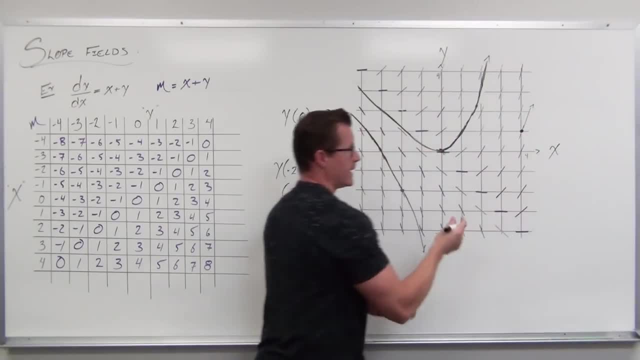 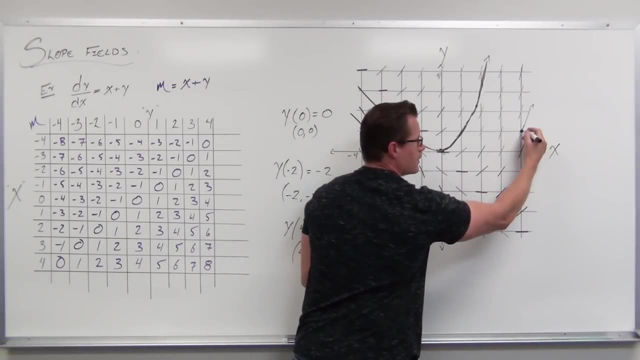 going to have to do this along that And it's going to be increasing slope after that. But before, remember that we have this asymptote thing. I'm trying to fit between my slopes here. I know that from here to here I go a slope of 0 to 1.. 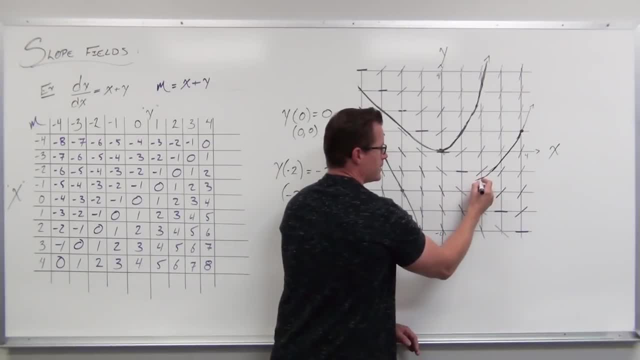 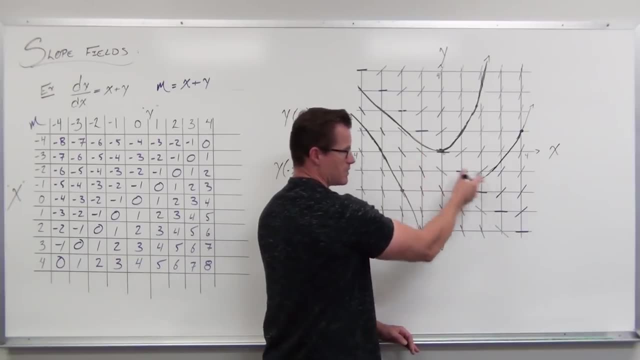 So I'm trying to make that pretty close to between there. Then, somewhere in here, I'm changing from this positive to a negative slope as I'm going backwards. So I'm going to hit a slope of 0. And then I have this asymptote that I got to get. 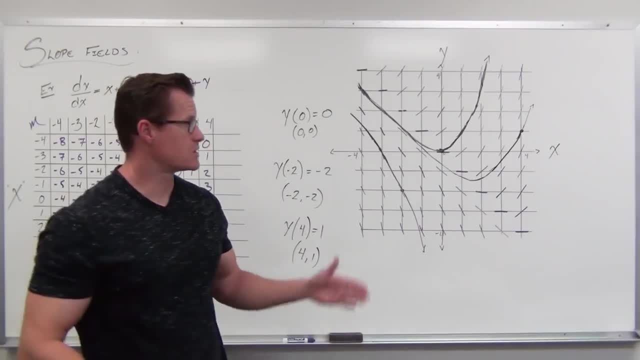 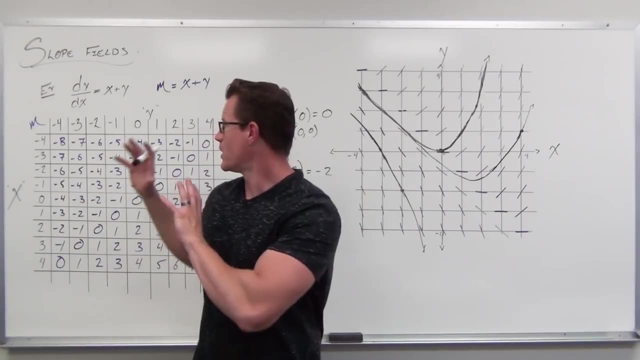 And that gives us our particular solution. that would have to go through that point. It's pretty cool because we can model these approximations without doing any real hardcore math. We know that our particular solution has to fit these slopes. That's what the slope field. 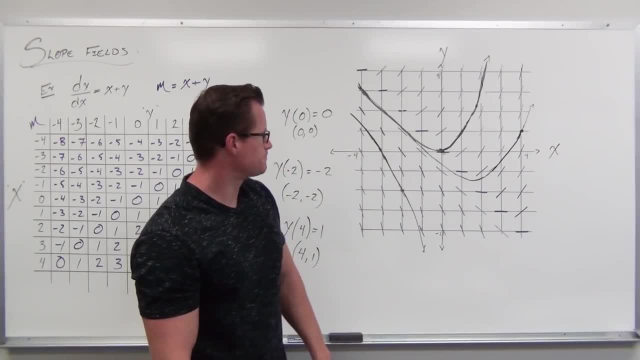 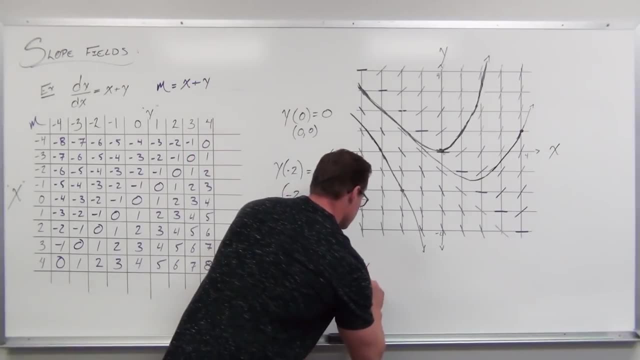 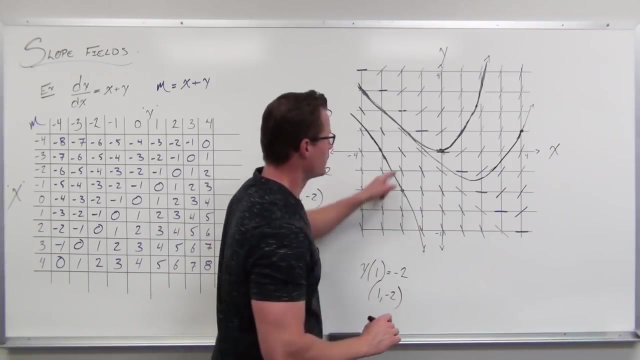 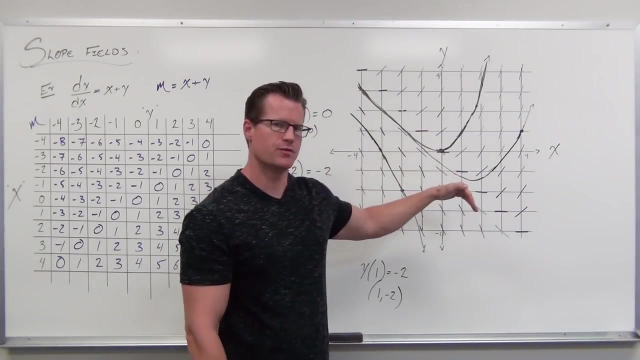 tells you It says it's got to fit here. Now one more question: What if I wanted to go through a point like 1 comma negative 2? 1 comma negative 2.. I am on that slope of negative 1.. I'm not changing as I'm going down that. 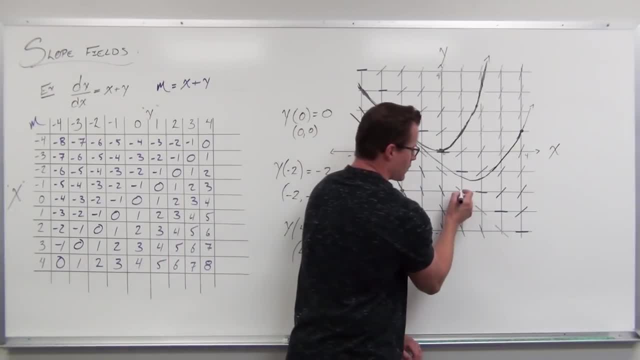 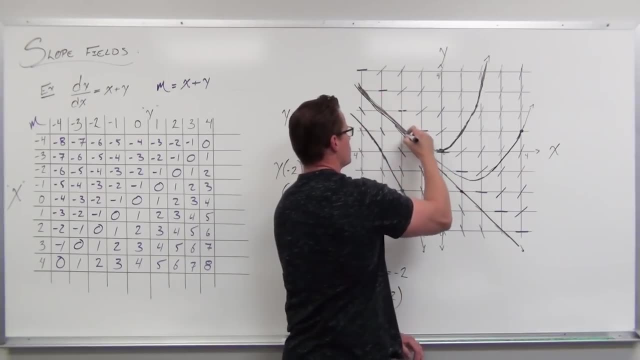 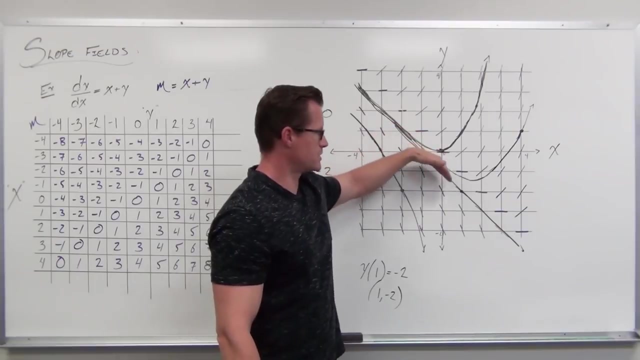 So on this particular point, before and after it, we're just traveling along that asymptote. And what that does? it says, yeah, if your slope is negative 1, as you move down that you're not changing, This slope is negative 1.. And I know we're only showing specific points here. 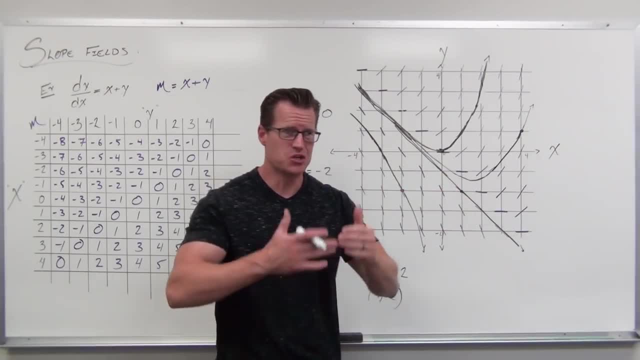 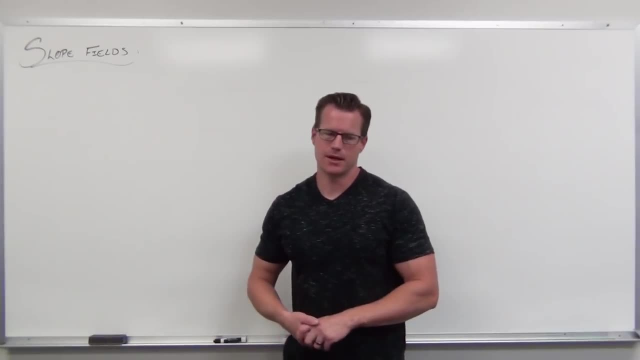 but every point between here would also have a slope of negative 1.. You can't get off of that. That's the asymptote. You're going to eventually be on that the whole entire time. So that's about it. That's how slope fields work. We take this differential equation that we may or 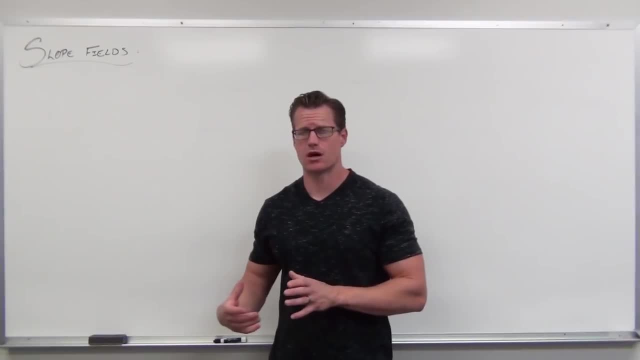 may not be able to solve And if we need to approximate it. so if you don't have a technique to solve it, we can create this Field that has a whole bunch of slopes at different points. Then we just have to find the particular solution that goes through a point and fits that slope field. So what you're getting 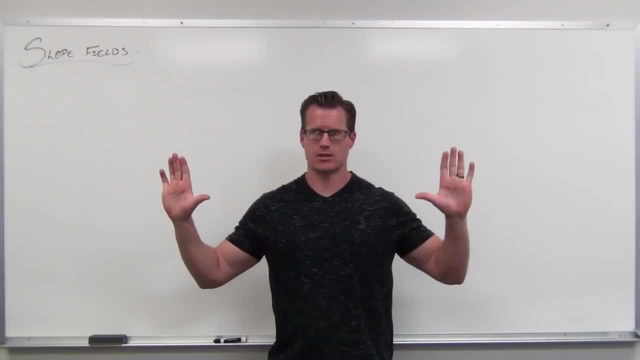 when you do a slope field is the general solution. That's why there's slopes everywhere And you go. well, there's not one curve that goes through all of those, Of course, because it won't even be a function To get a specific one particular function. you need a particular point. Then we 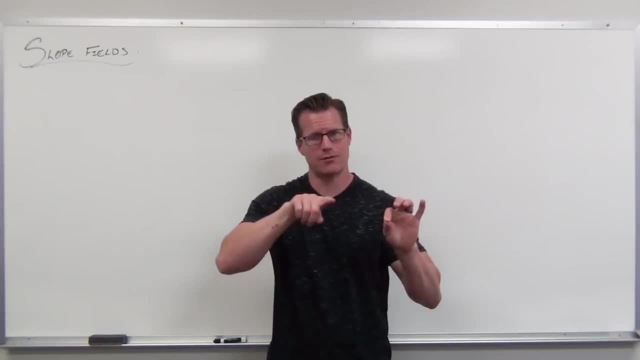 can match up from that point, fit all the slopes before and after that. So just notice that on the previous example, I know we're only we're only doing one. It just takes a long time and there's nothing different about any of these things that you do. 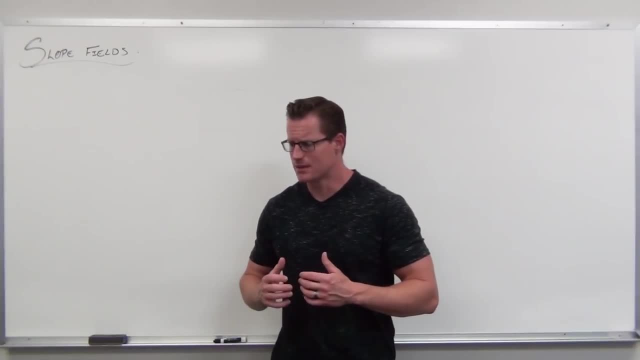 So just follow the same exact process. Just notice that how, given that if you have a point, a particular solution, it gives you a unique solution to that differential equation. All the paths through the slope field are solutions to that particular differentially range of liquid time. So all of all the different curves you could draw, So every single one of them.